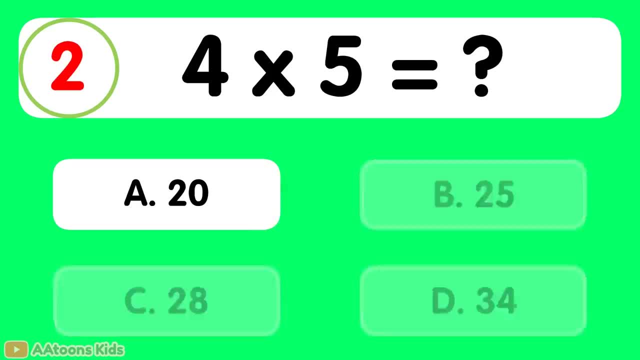 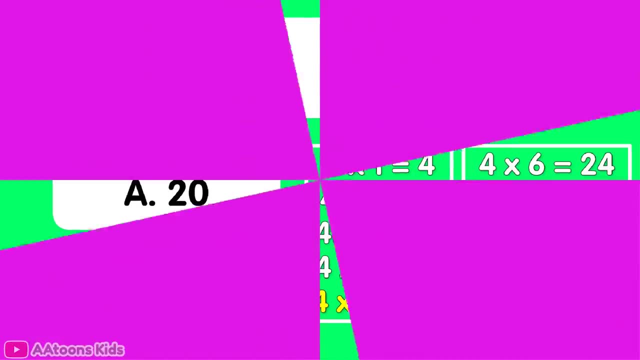 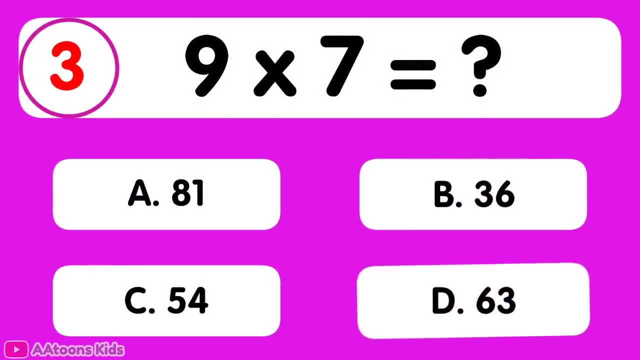 25,, 26,, 27,, 28,, 29,, 30,, 31,, 32,, 33,, 34,, 35,, 36,, 37,, 38,, 39,, 40,, 41,, 42,, 43,, 44,, 45,. 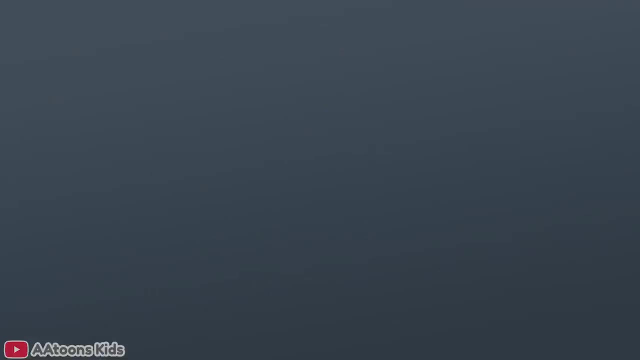 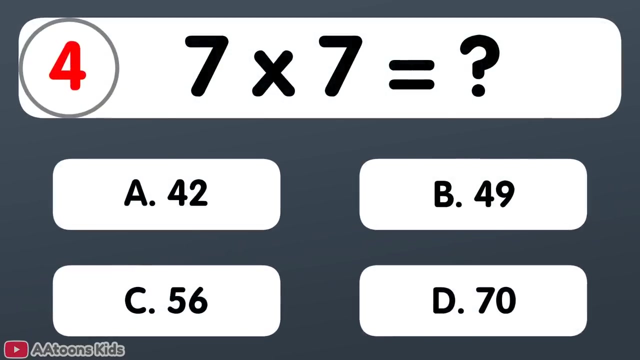 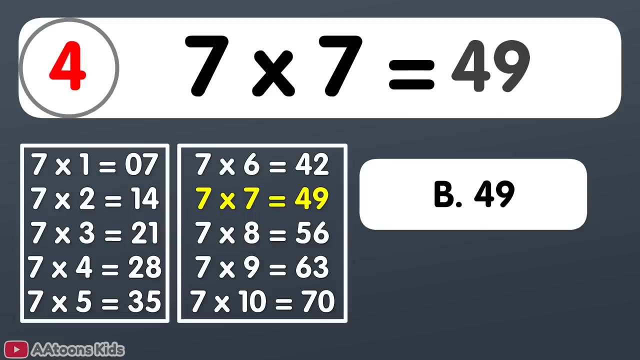 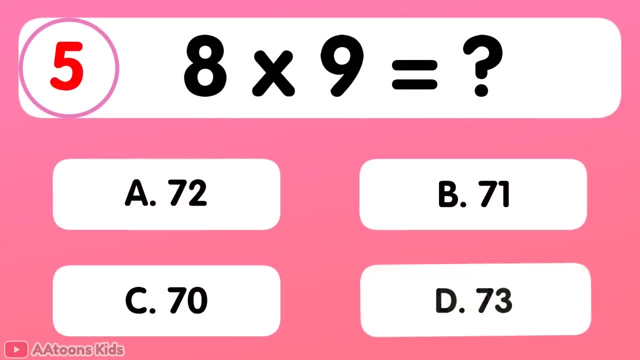 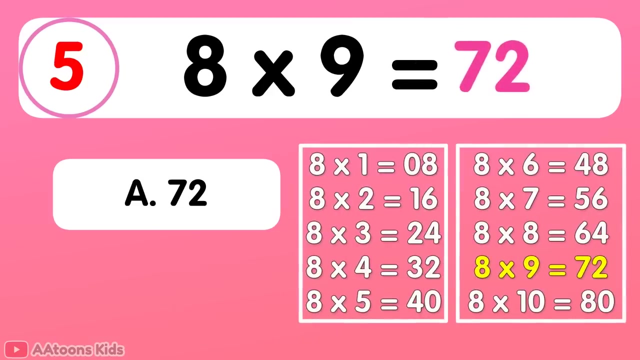 43.. 7 times 7 is equal to 49.. 7 times 7 is 49.. 8 times 9 is equal to 49.. 72.. 8 times 9 is 72.. 10 times 3 is equal to. 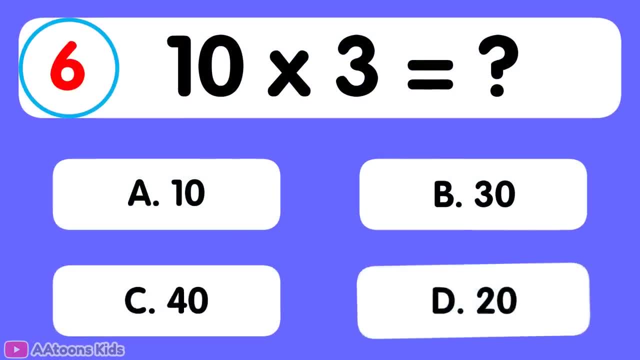 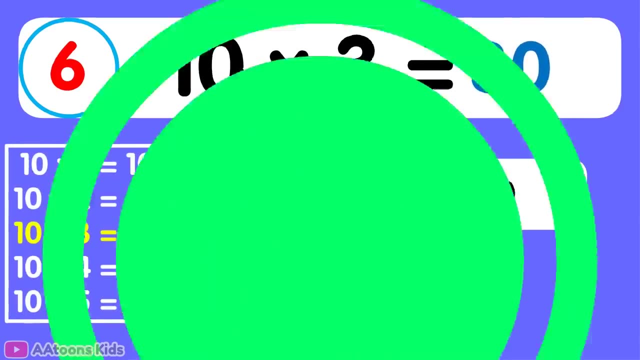 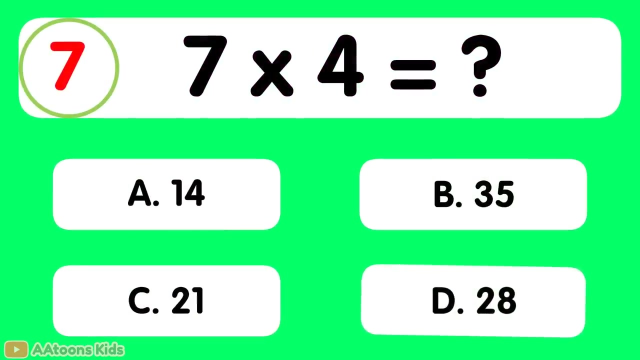 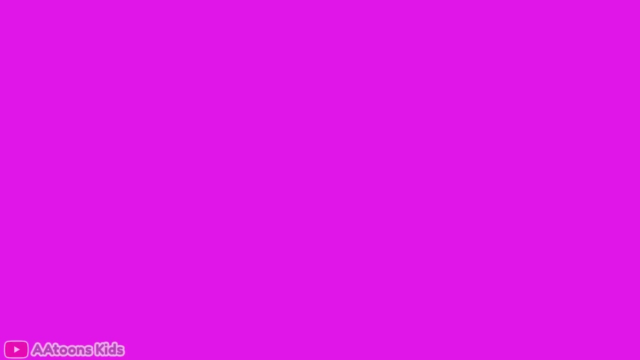 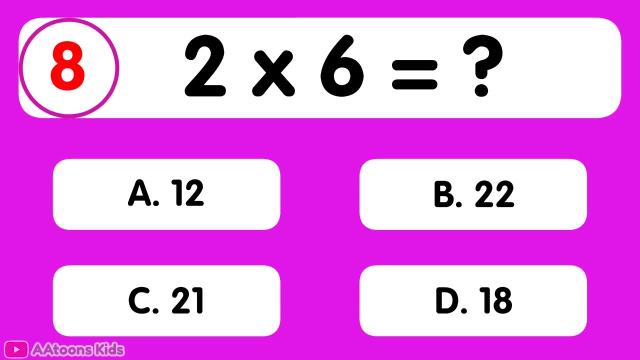 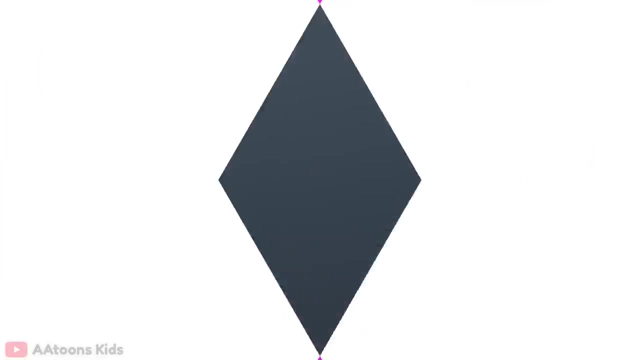 39.. 72.. 10 x 3 is 30. 7 x 4 is equal to 28. 7 x 4 is 28. 2 x 6 is equal to 12. 2 x 6 is 12. 8 x 7 is equal to. 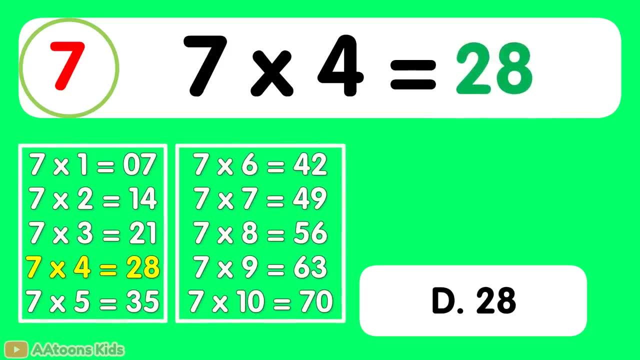 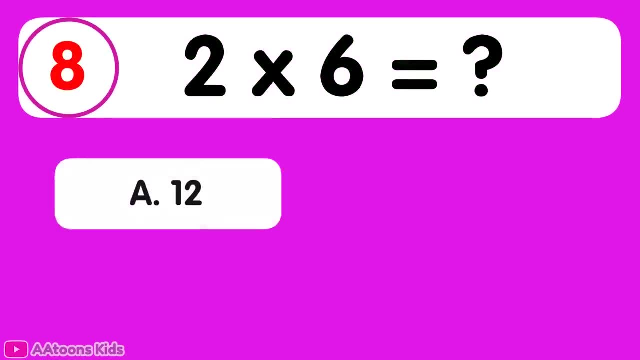 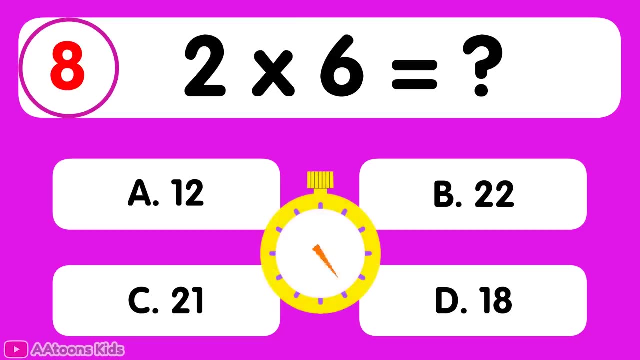 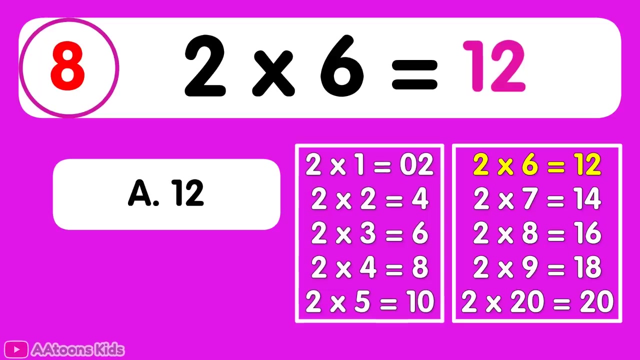 27.. 8 times 6 is equal to 7.. You can Probably tell now that you know what 10 is Then점. 4 times 7 is equal to 2 × 6 is equal to 12. 2 × 6 is 12. 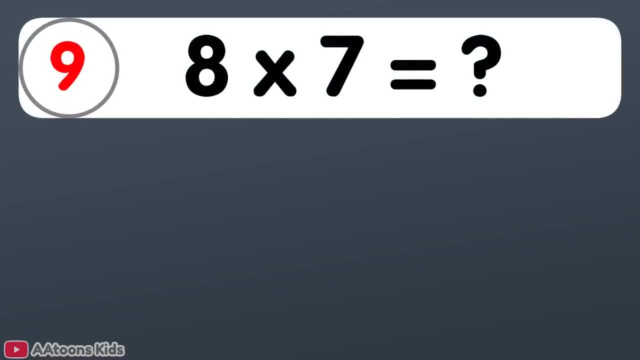 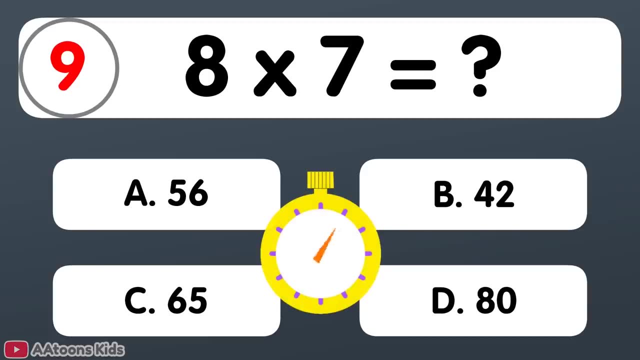 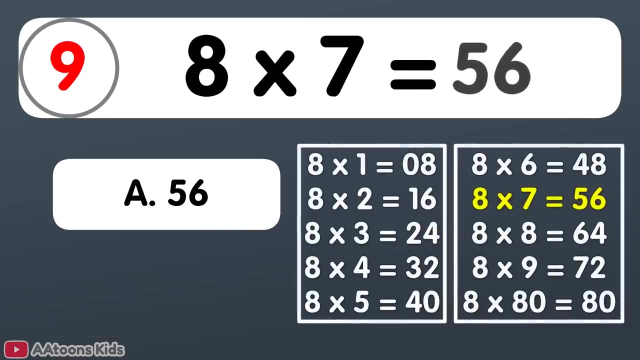 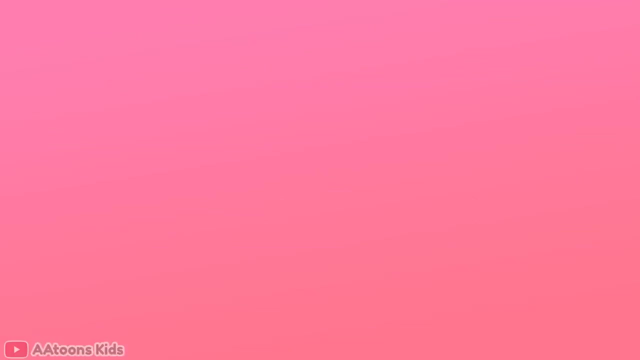 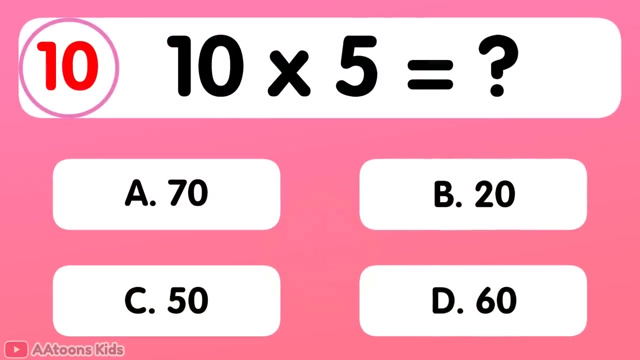 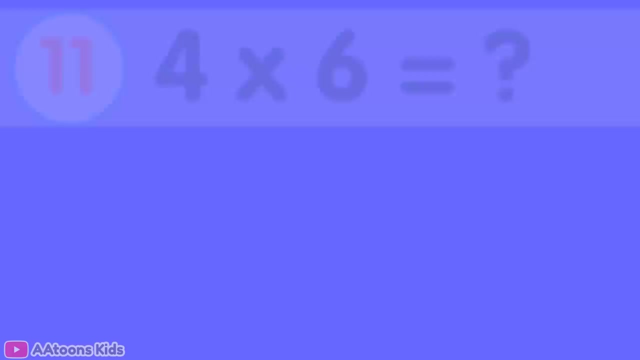 8 × 7 is equal to 56. 8 × 7 is 56. 10 × 5 is equal to. 10 × 5 is equal to: 10 × 5 is 50. 10 × 5 is 50. 4 × 6 is equal to. 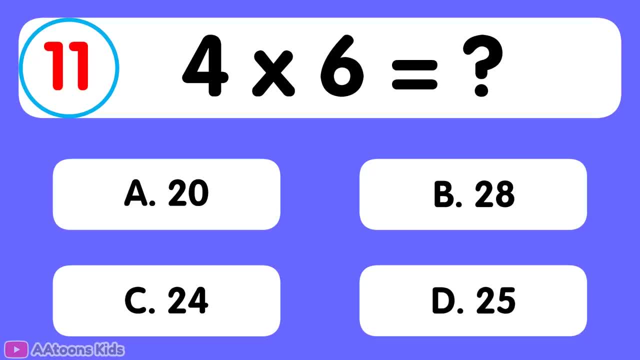 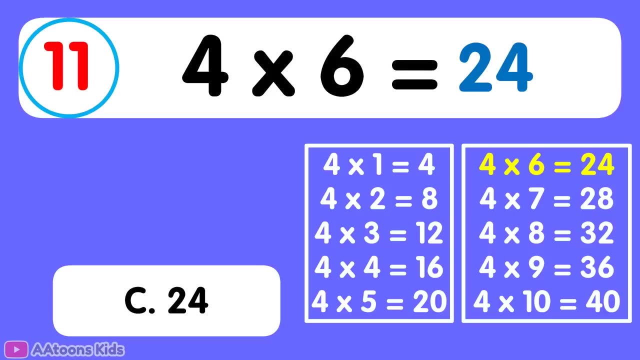 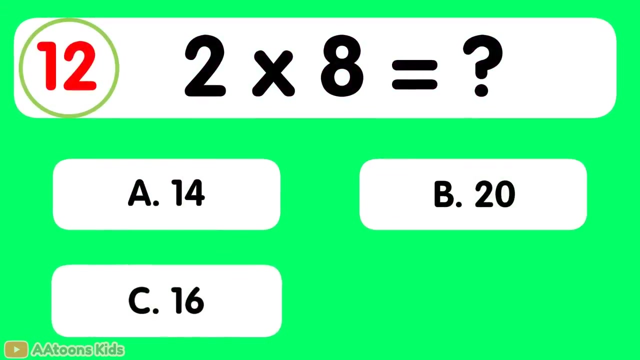 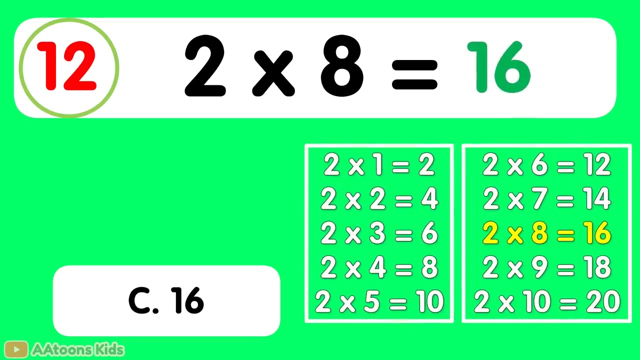 4 × 6 is equal to 24 × 6 is 24. 2 × 8 is equal to 8 × 6 is 24. 16 × 2 × 8 is 16. 16 × 2 × 8 is 16. 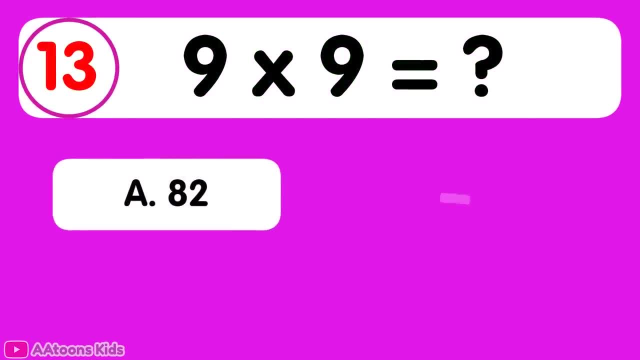 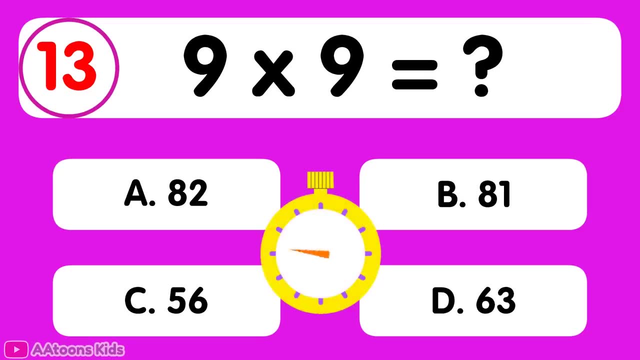 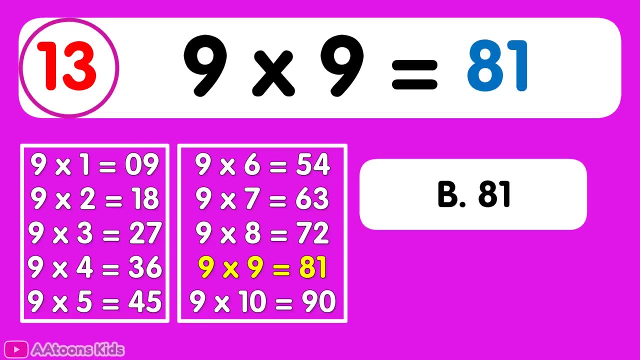 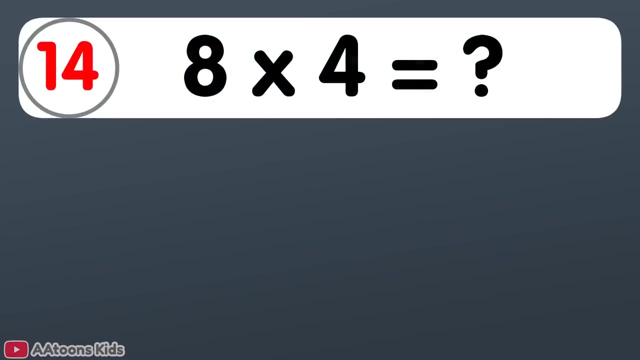 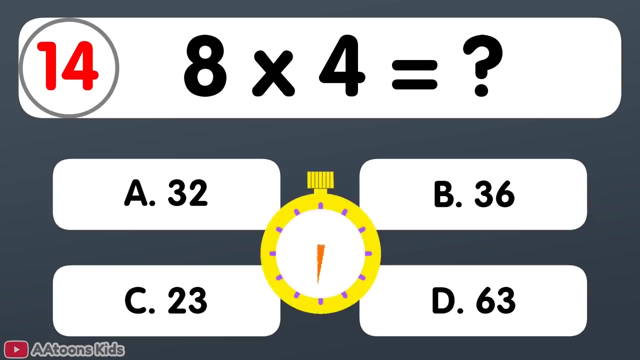 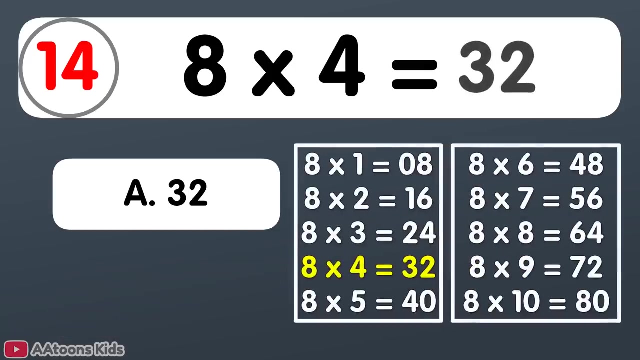 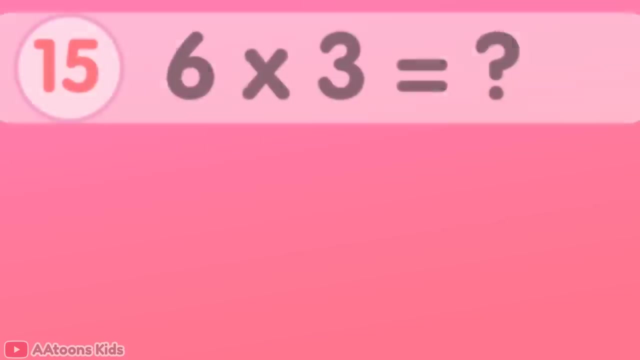 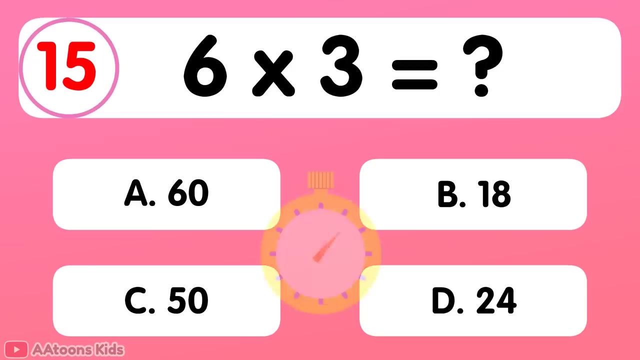 9 times 9 is equal to 81. 9 times 9 is 81. 8 times 4 is equal to 32. 8 times 4 is 32. 6 times 3 is equal to 18. 6 times 3 is 18. 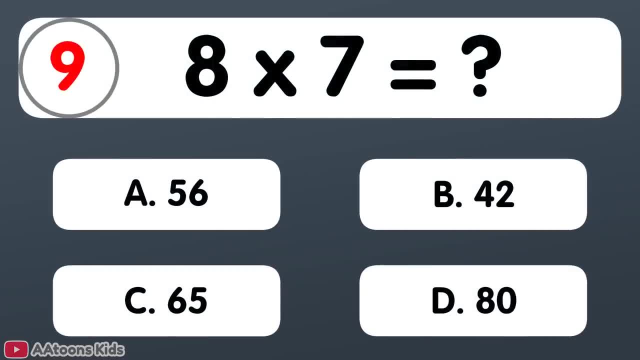 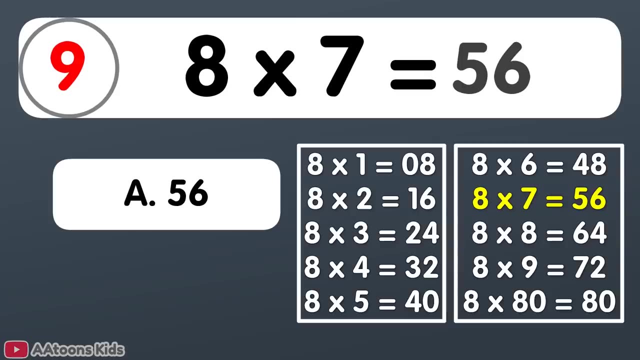 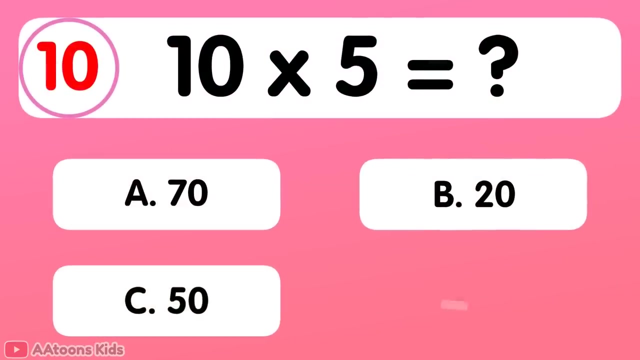 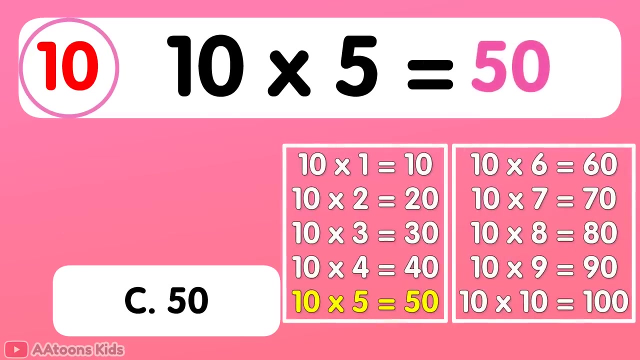 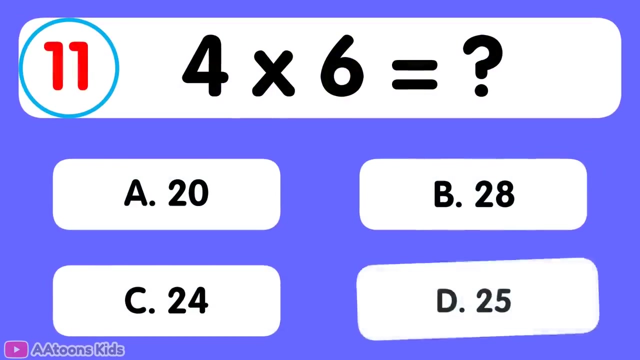 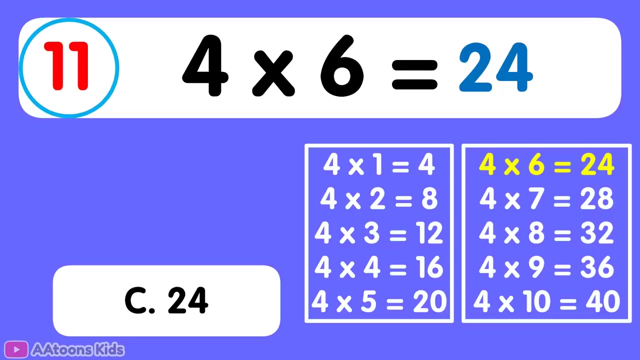 56. 8 x 7 is 56. 10 x 5 is equal to 50. 10 x 5 is 50. 4 x 6 is equal to 24. 4 x 6 is 24. 5 4 x 6 is 24. 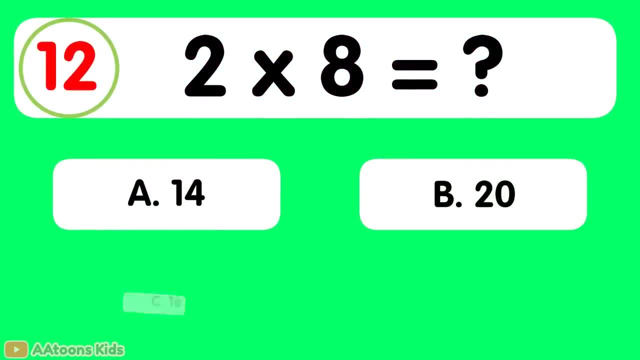 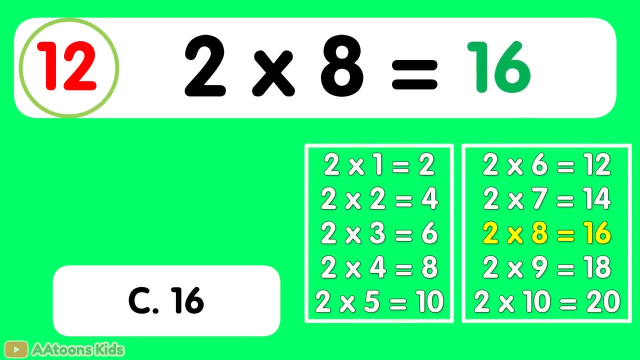 2, 8 x 7 is 21, 16, 2 x 8 is 7, 6 x 7 is 22, 2, 8 x 7 is 21, 2, 8 x 9 is 18, 8 x 9 is 20. 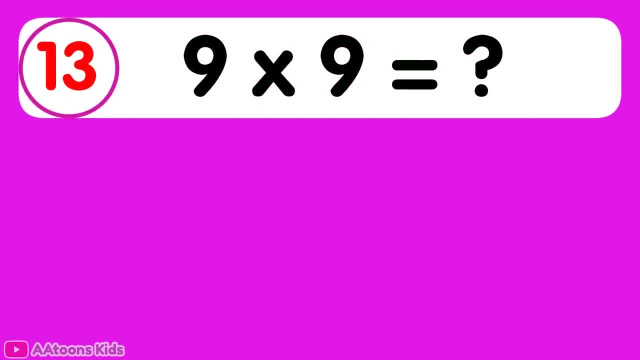 1 x 9 is 21, 2, 8 x 10 is 14. 2, 8 x 1 is 11. 2, 8 x 2 is 24. 2, 8 x 17 is 51. 2, 8 x 1 is 13. 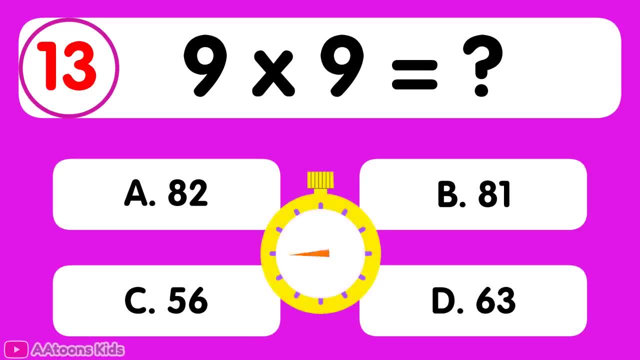 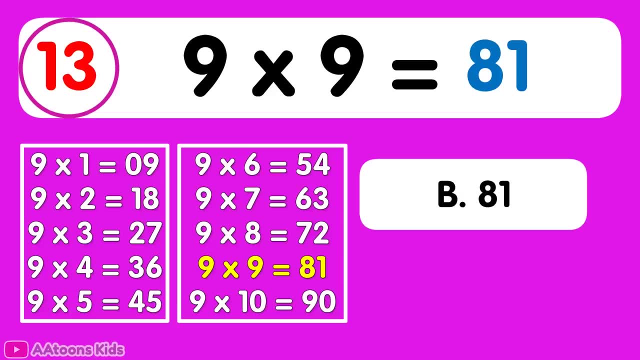 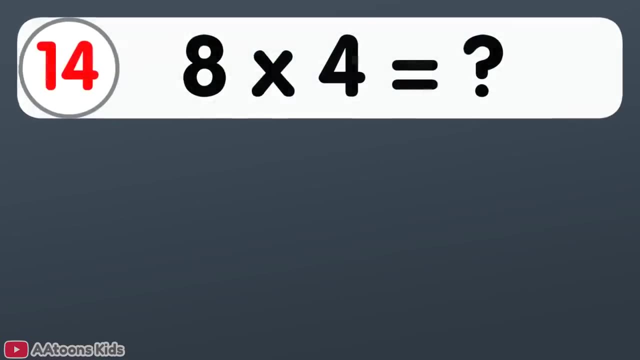 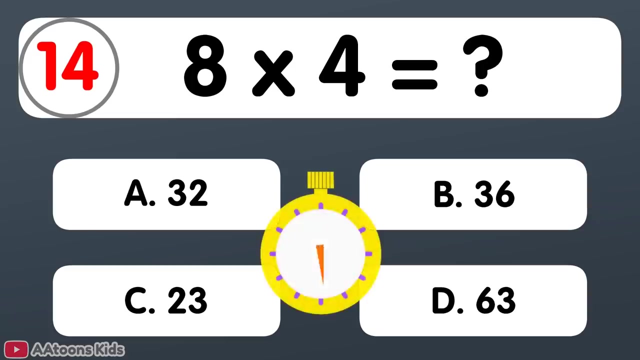 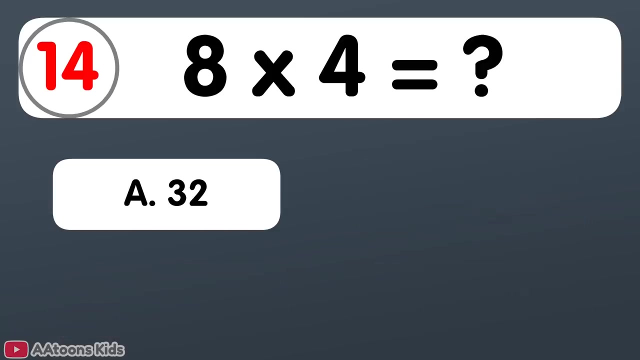 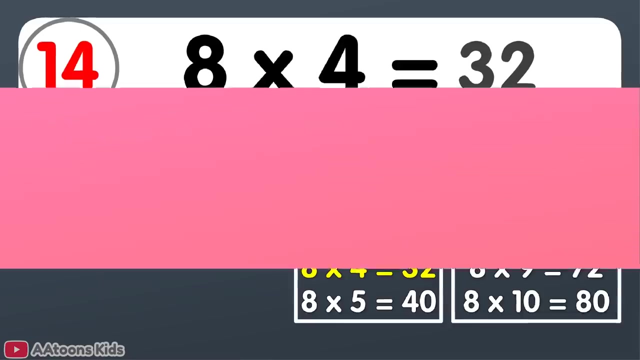 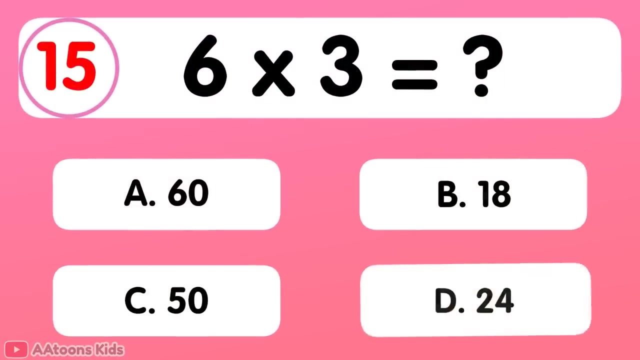 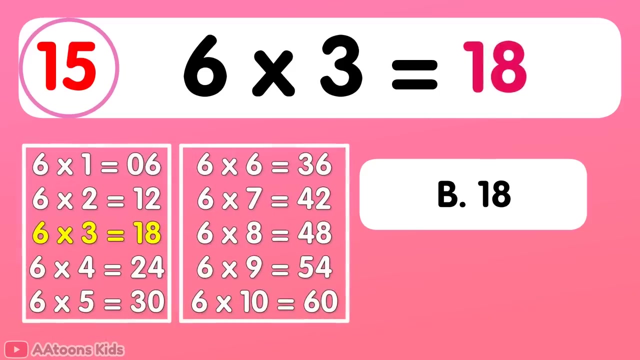 2, 8 x 9 is 14, 81,. 9 times 9 is 81. 8 times 4 is equal to 32,. 8 times 4 is 32. 6 times 3 is equal to 80,. 6 times 3 is 80. 2 times 9 is equal to. 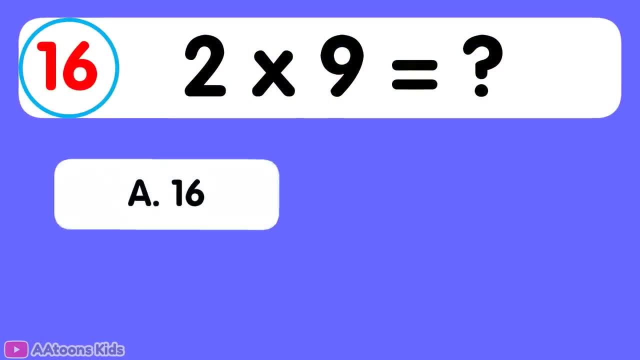 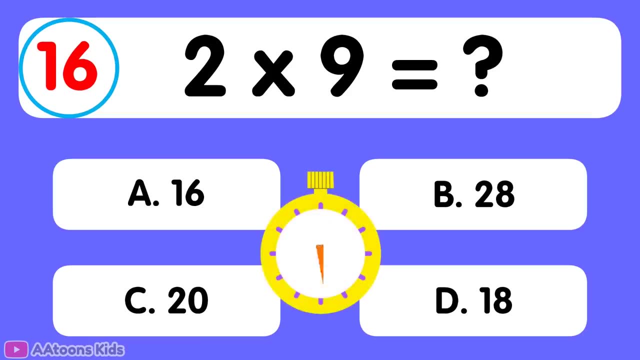 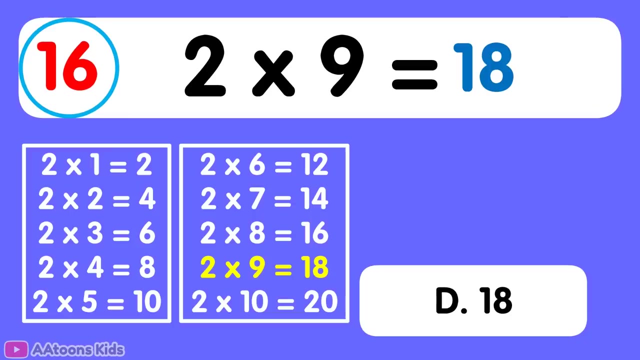 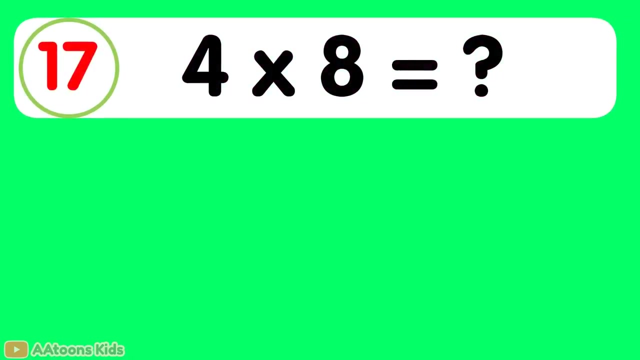 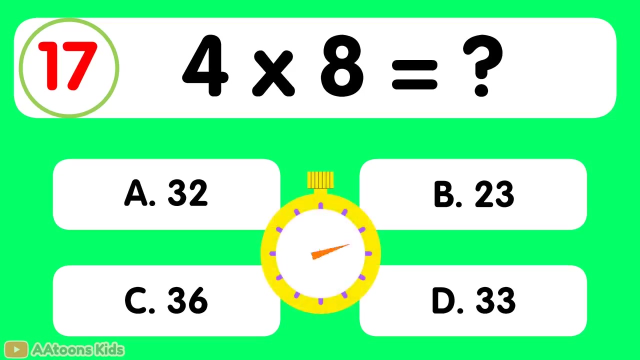 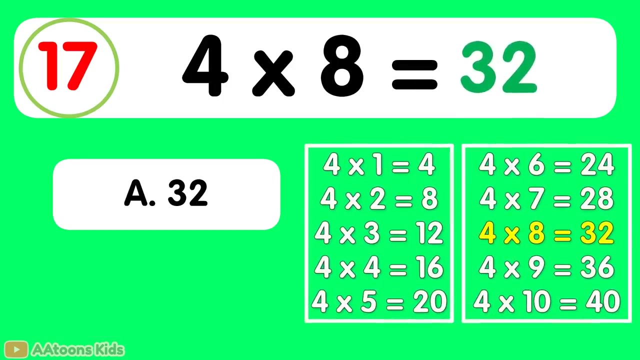 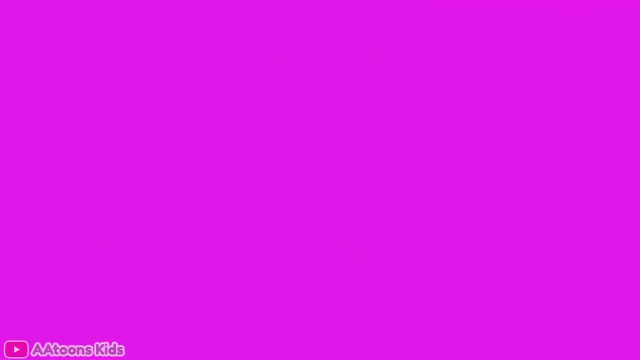 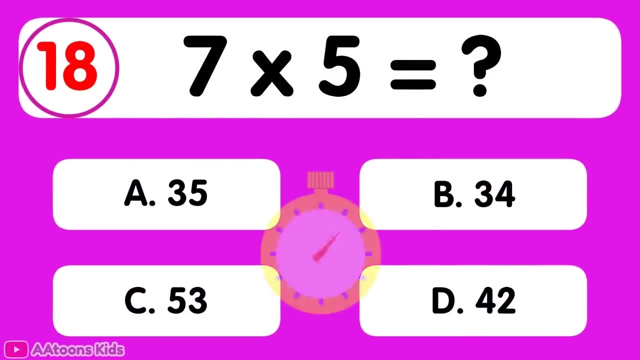 2 times 9 is equal to 18. 2 times 9 is 18. 4 times 8 is equal to 32. 4 times 8 is 32. 7 times 5 is equal to 35. 7 times 5 is 35. 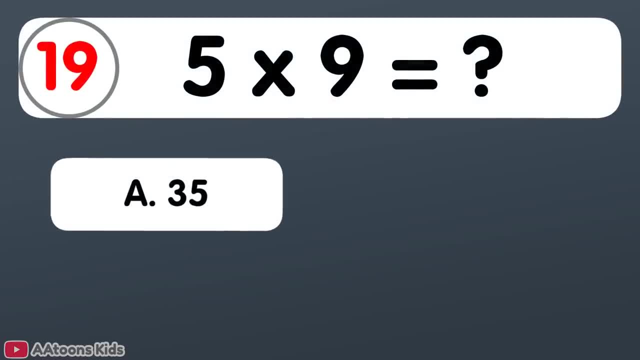 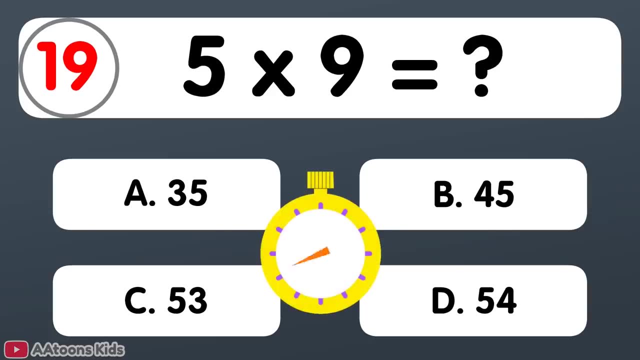 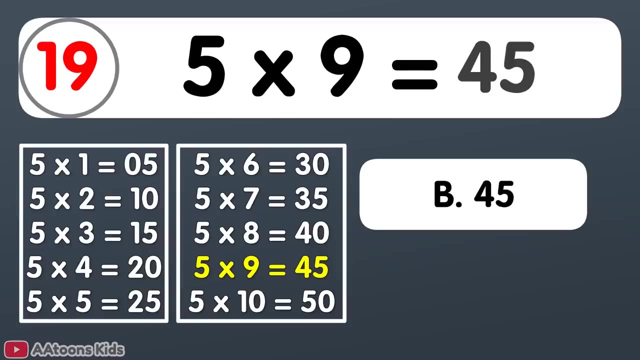 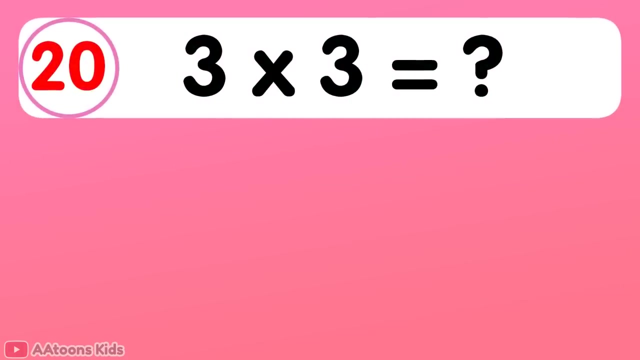 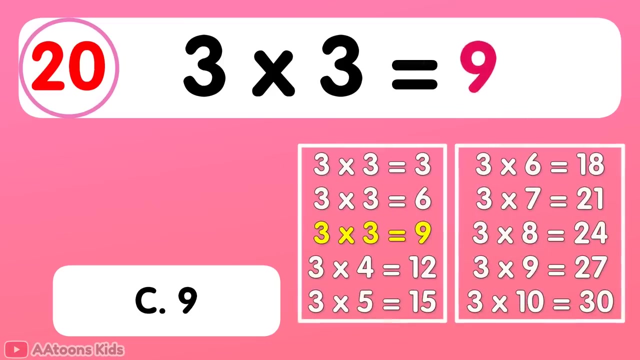 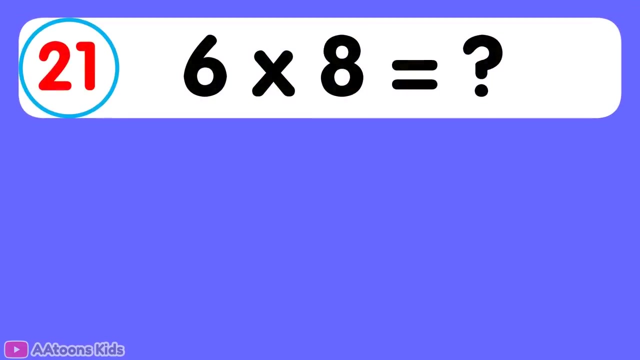 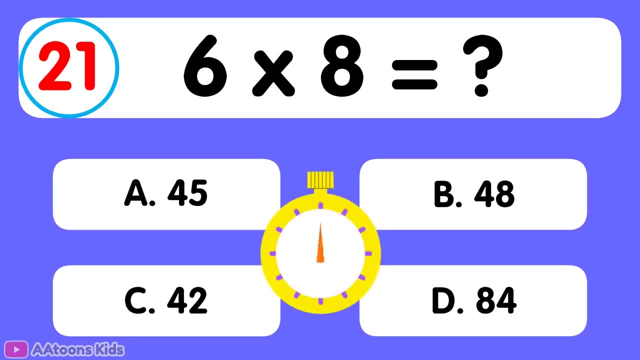 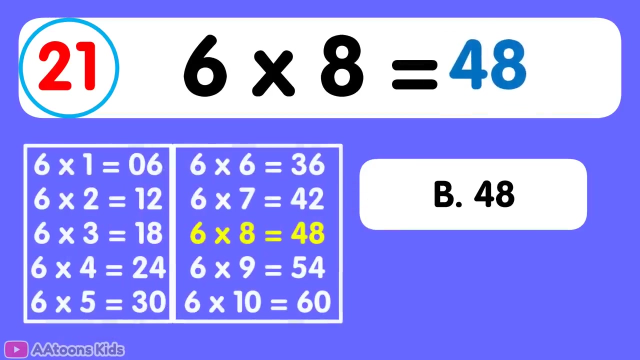 5 times 9 is equal to 45. 5 times 9 is 45. 3 times 3 is equal to 9. 3 times 3 is 9. 6 times 8 is equal to 48. 6 times 8 is 48. 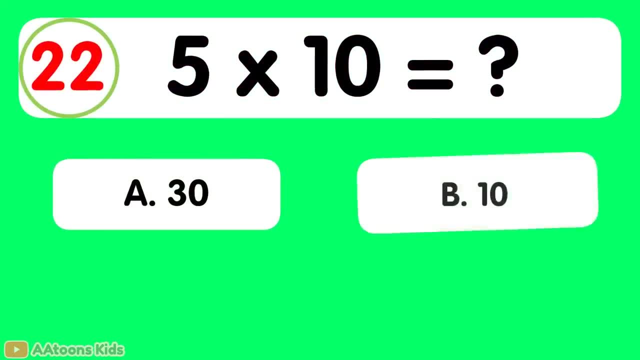 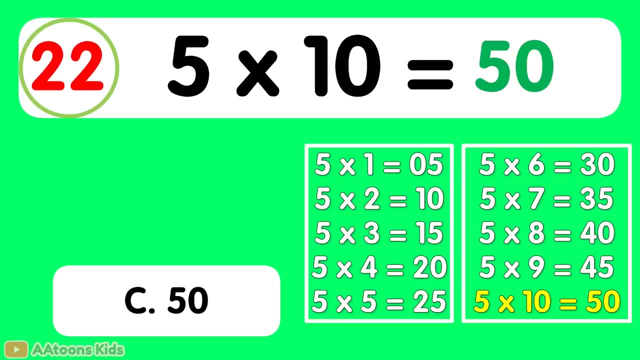 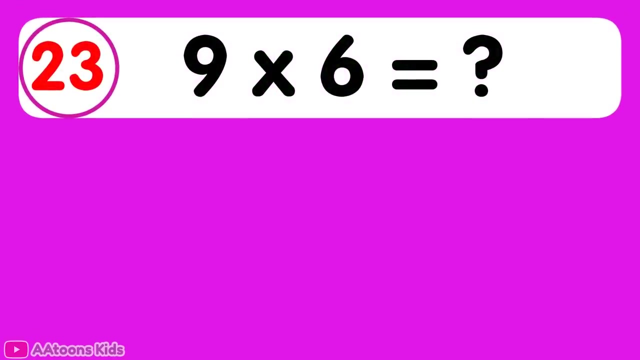 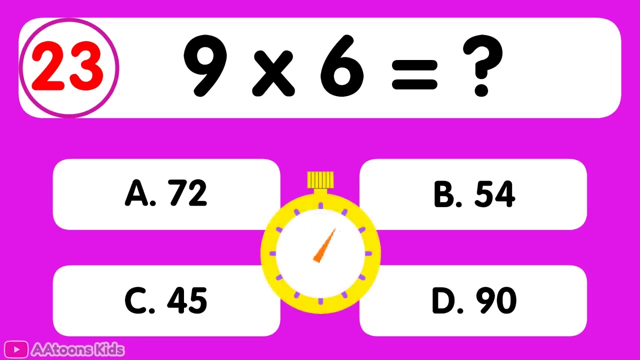 5 times 10 is equal to 33, 50. 5 times 10 is 50. 9 times 6 is equal to 54. 6 times 9 is equal to 26. 3 times 6 is equal to 23, 36. 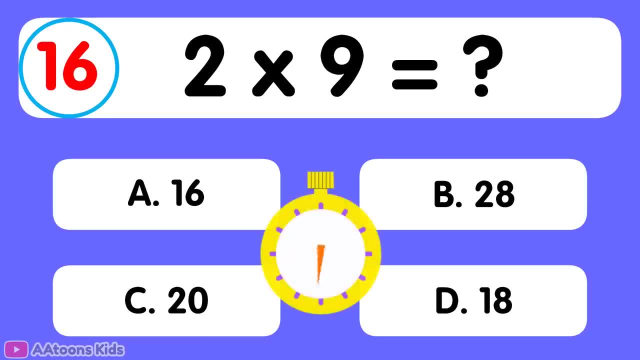 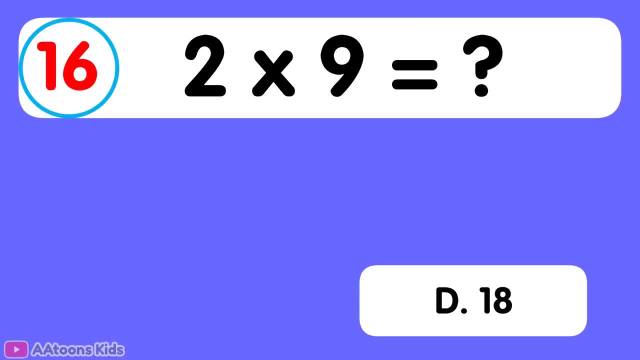 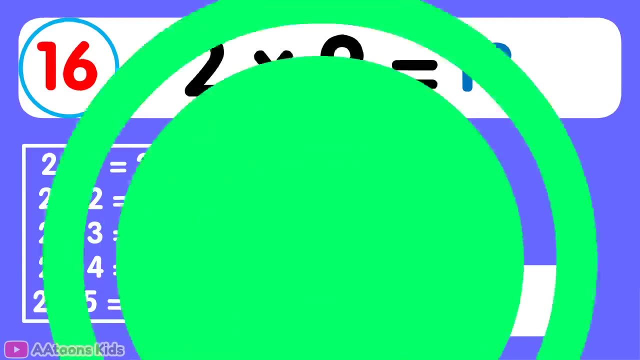 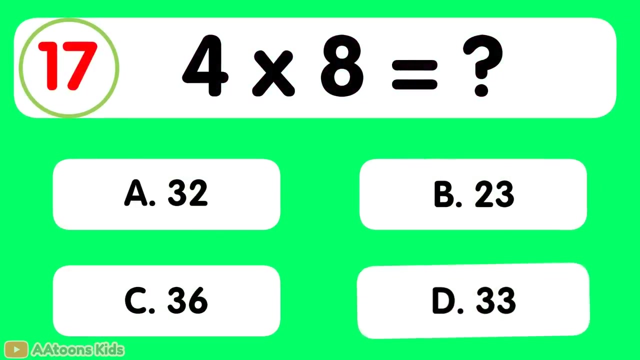 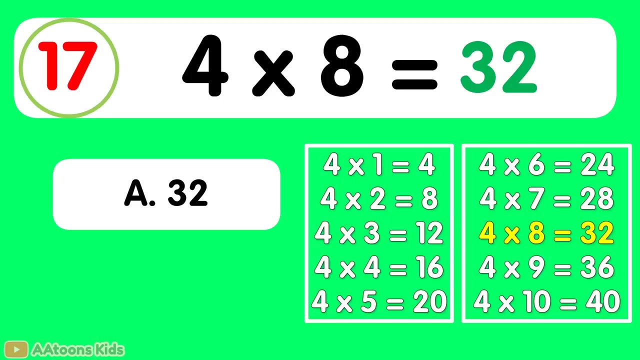 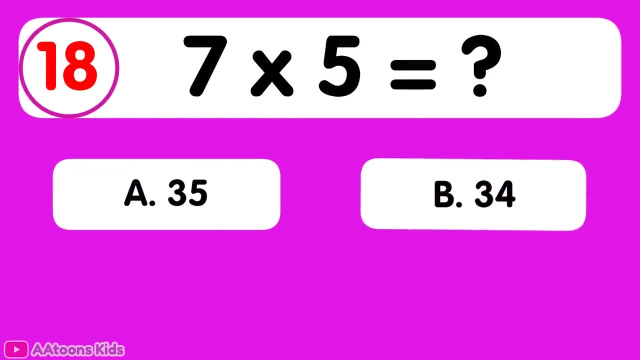 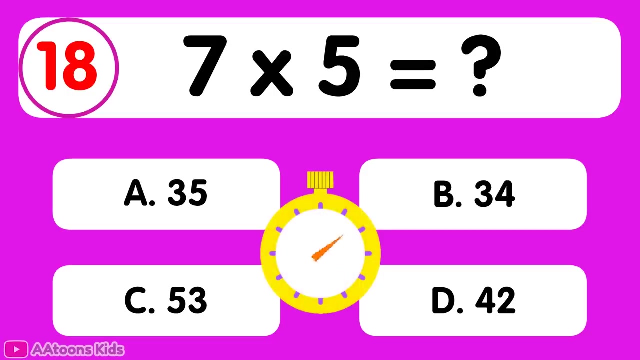 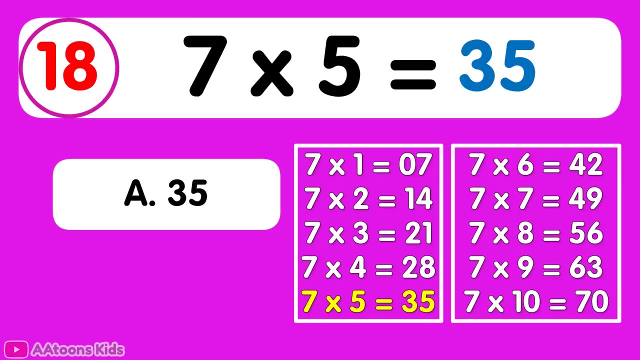 18,2 times 9 is 18,. 2 times 9 is 18. 18. 4 times 8 is equal to 32. 4 times 8 is 32. 7 times 5 is equal to 35. 7 times 5 is 35. 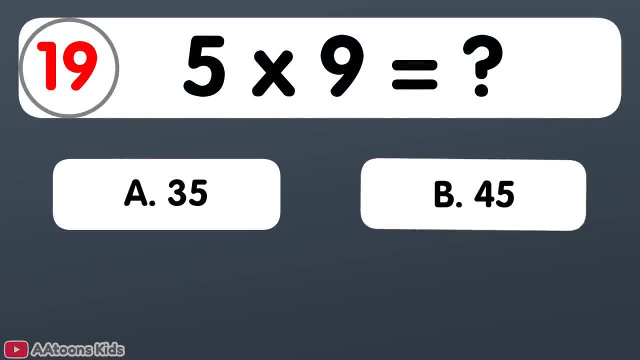 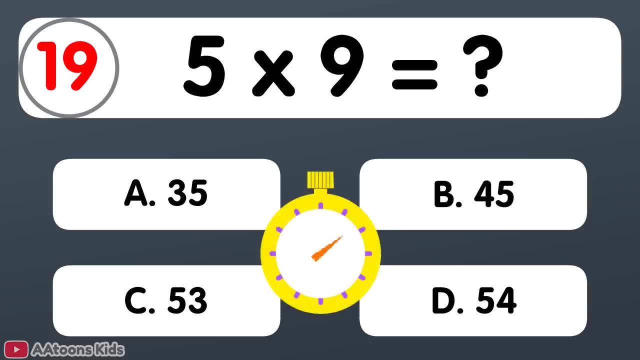 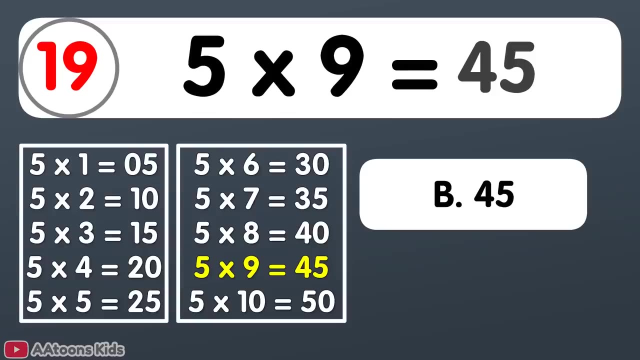 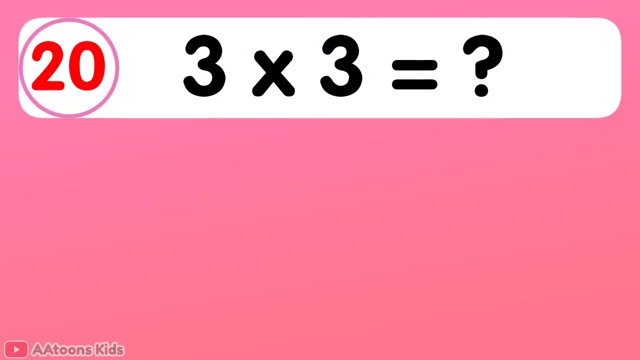 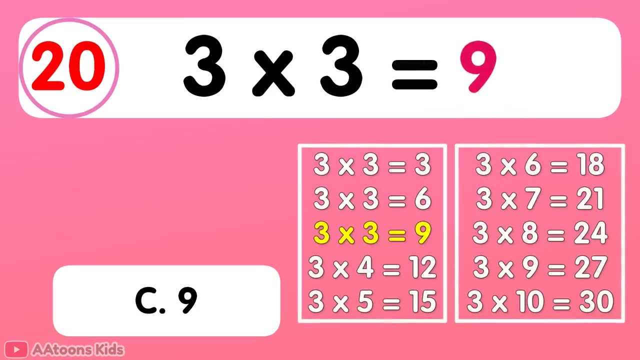 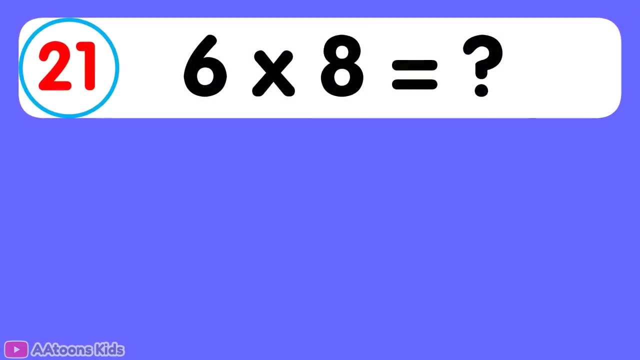 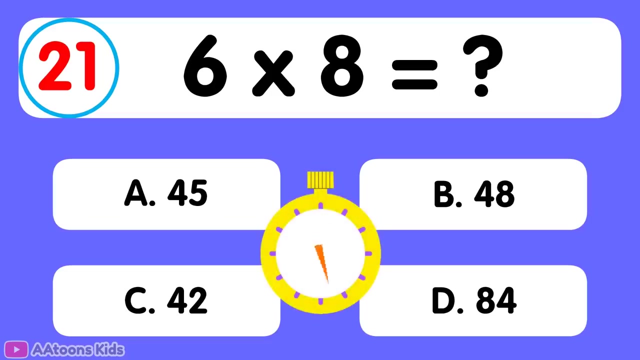 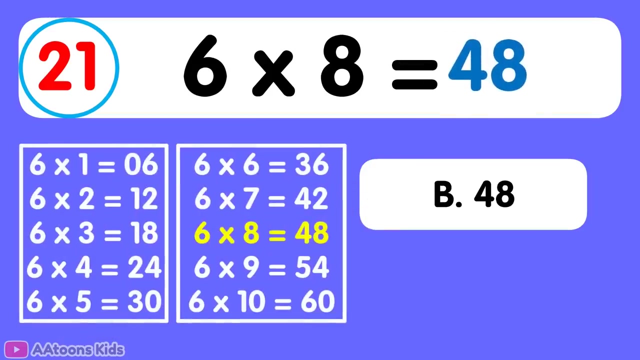 5 times 9 is equal to 45. 5 times 9 is 45. 3 times 3 is equal to 9.. 3 times 3 is 9.. 6 times 8 is equal to 48.. 6 times 8 is 48.. 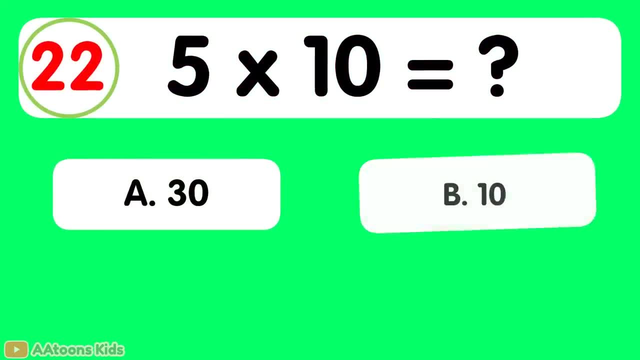 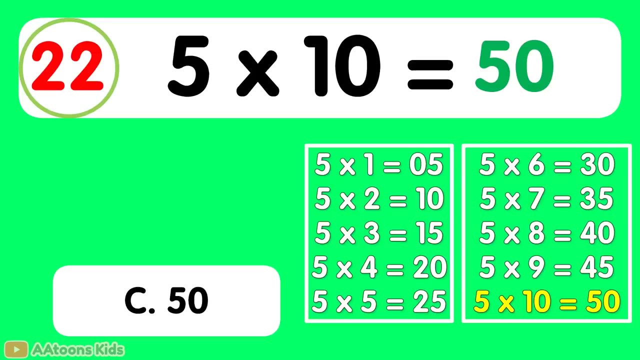 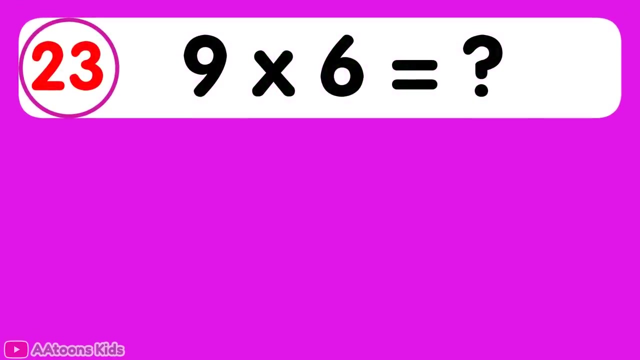 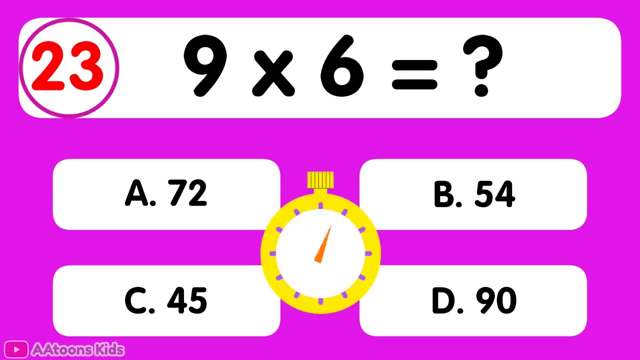 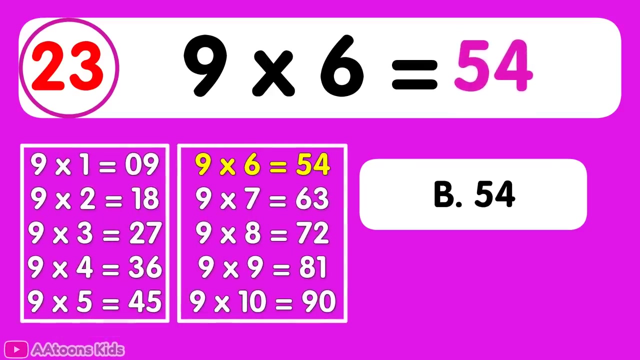 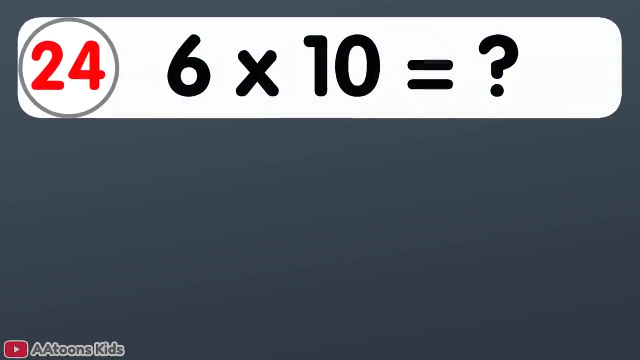 5 times 10 is equal to 50.. 5 times 10 is 50.. 9 times 6 is equal to 54.. 9 times 6 is 54.. 6 times 10 is equal to 64.. 6 times 10 is equal to. 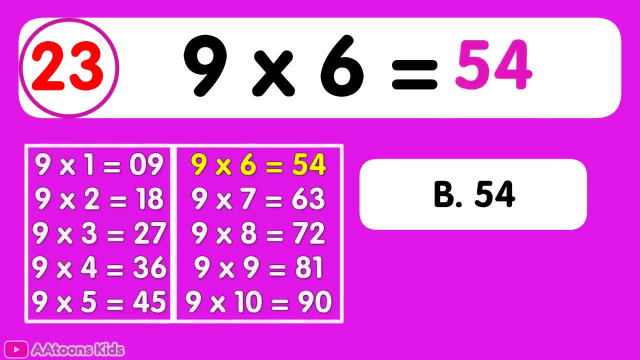 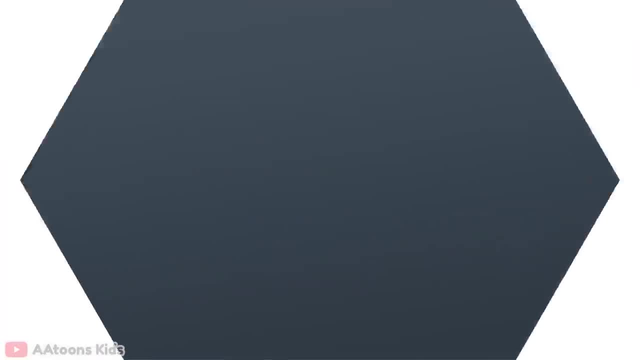 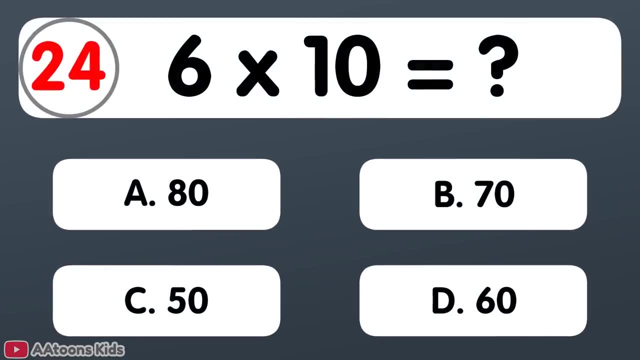 7 times 9 is equal to 37. 5 times 7 is equal to 36, 54.. 9 times 6 is 54.. 6 times 10 is equal to 60.. 6 times 10 is 60.. 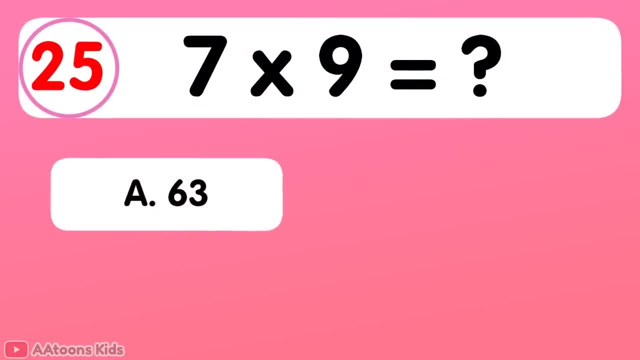 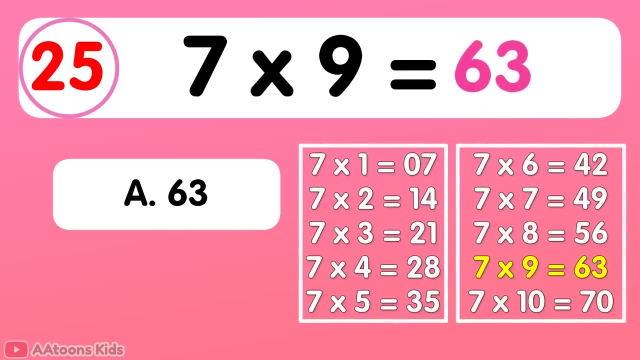 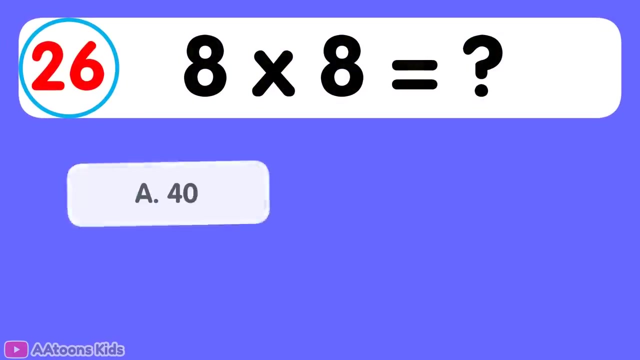 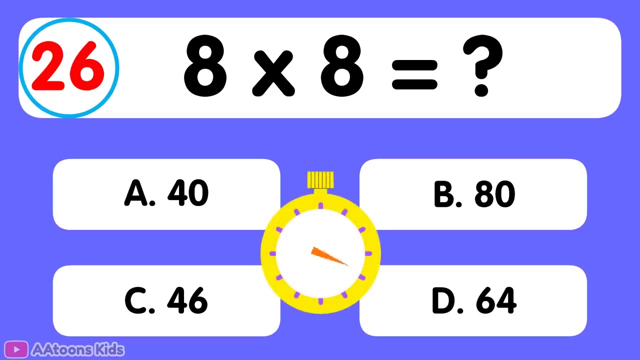 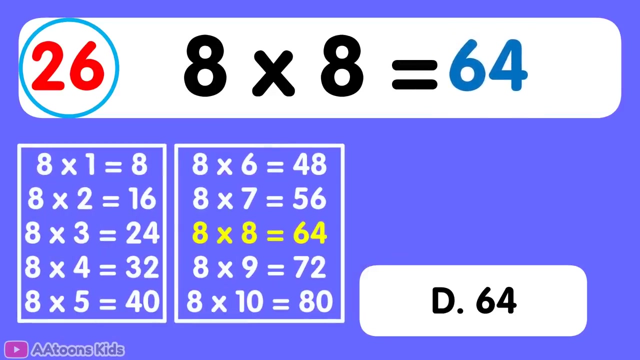 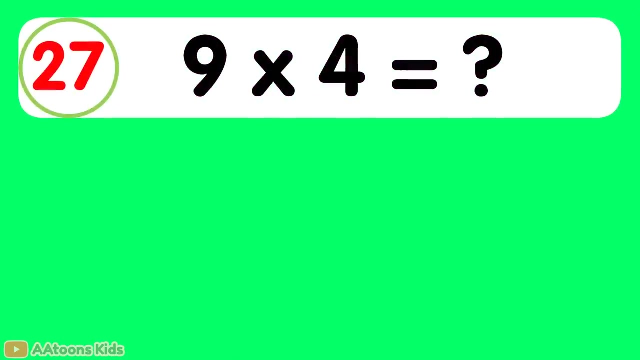 7 times 9 is equal to 63.. 7 times 9 is 63.. 8 times 8 is equal to 63.. 64.. 8 times 8 is 64.. 9 times 4 is equal to. 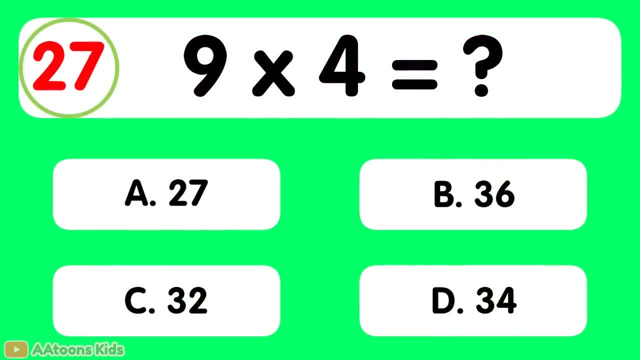 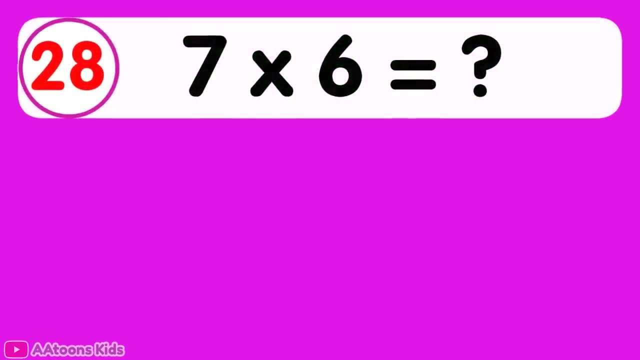 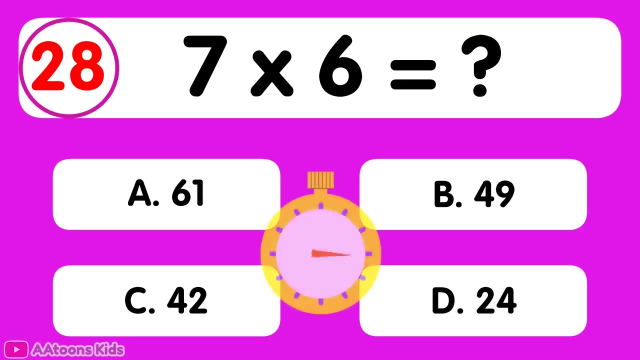 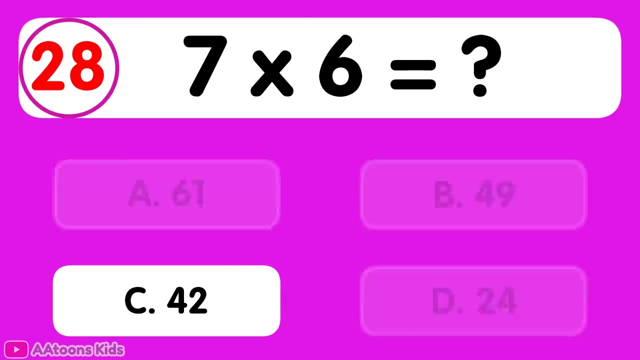 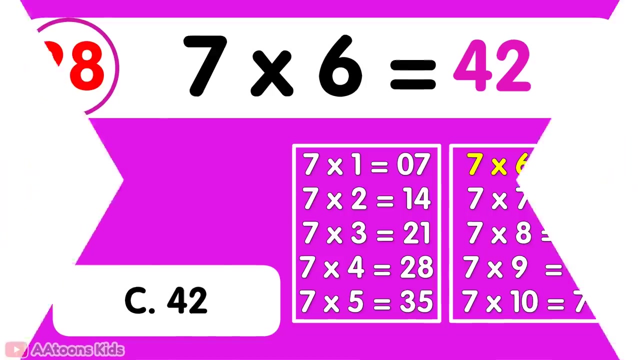 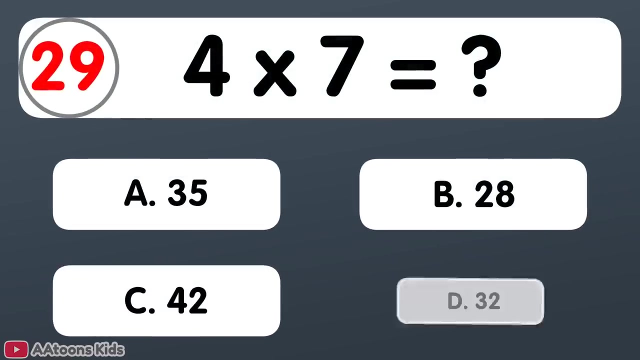 64.. 36.. 7 times 6 is equal to 42.. 7 times 6 is 42.. 4 times 7 is equal to 2 times 7 is equal to 28.. 4 times 7 is meaning. 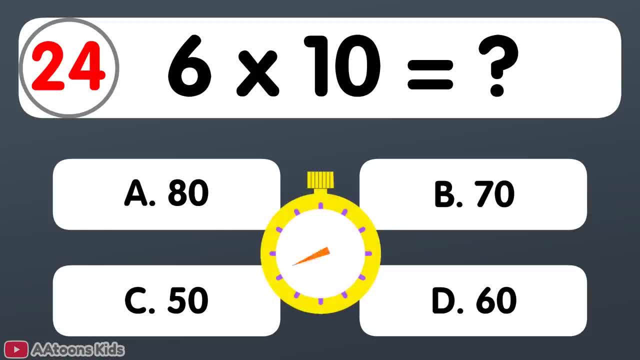 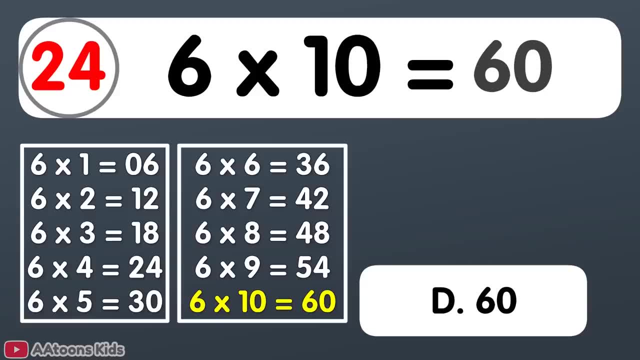 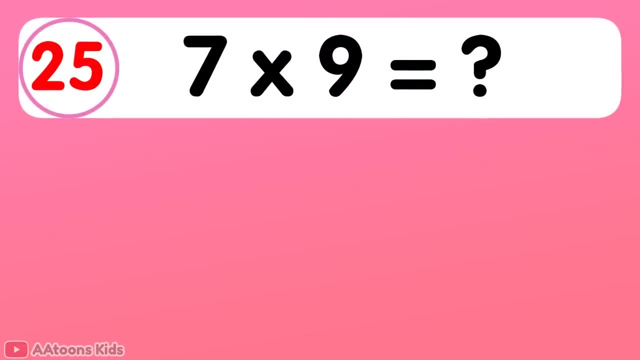 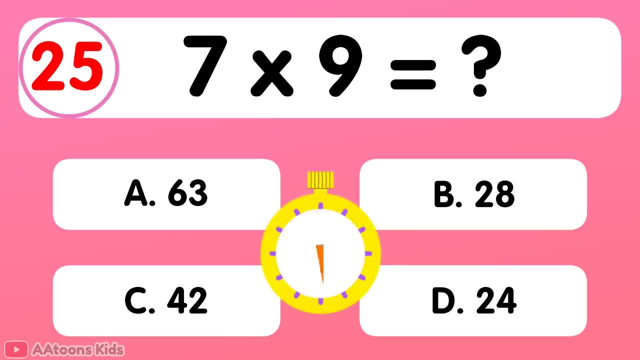 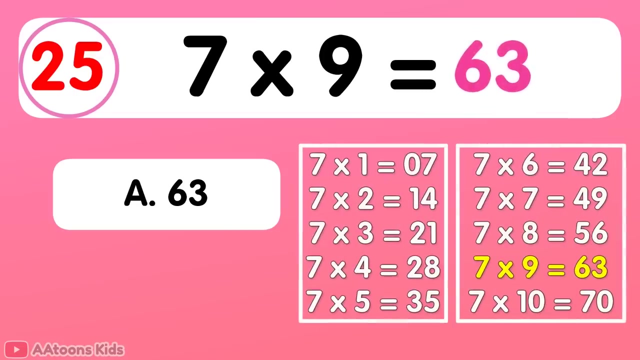 55.. 6 times 10 is equal to 55.. 6 times 10 is equal to 60.. 6 times 10 is 60.. 7 times 9 is equal to 63.. 7 times 9 is 63.. 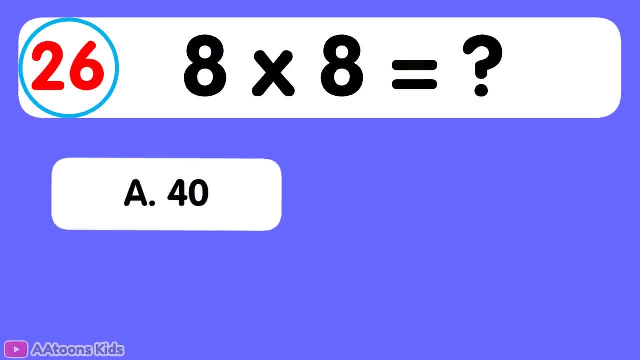 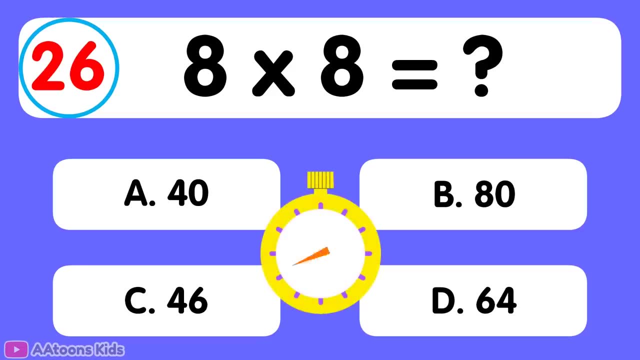 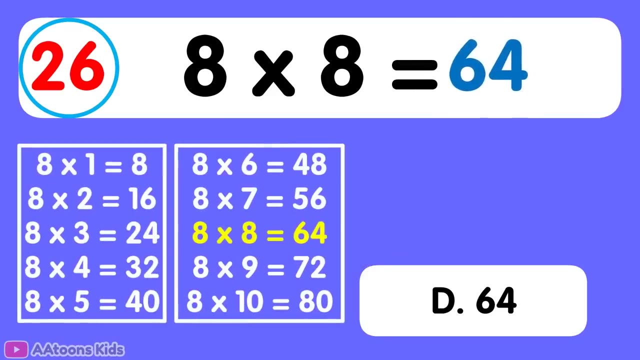 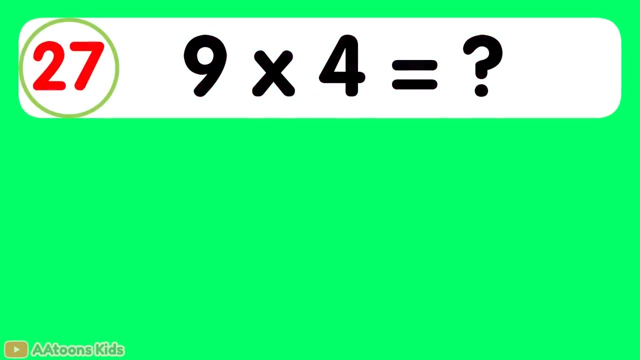 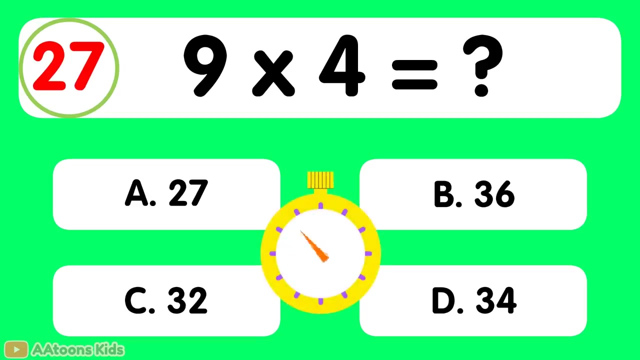 8 times 9 is 63.. 8 times 8 is equal to 64.. 8 times 8 is 64.. 9 times 4 is equal to 64.. 9 times 4 is equal to 66.. 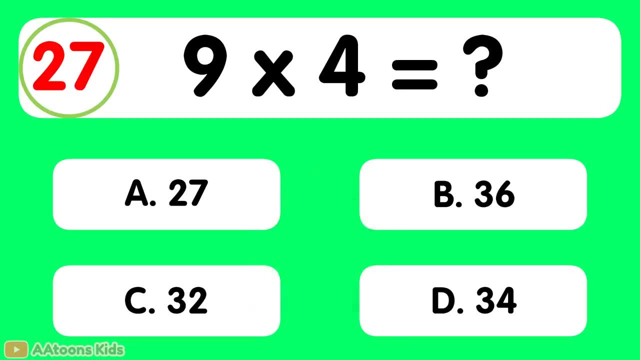 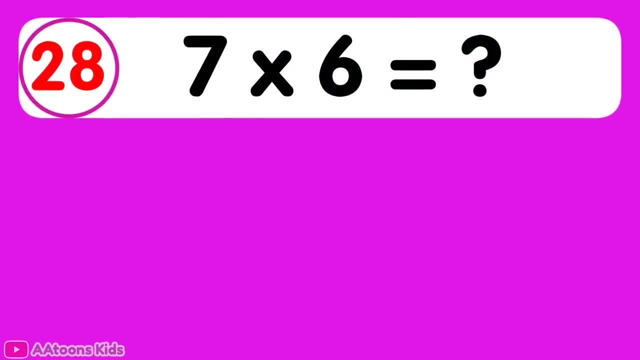 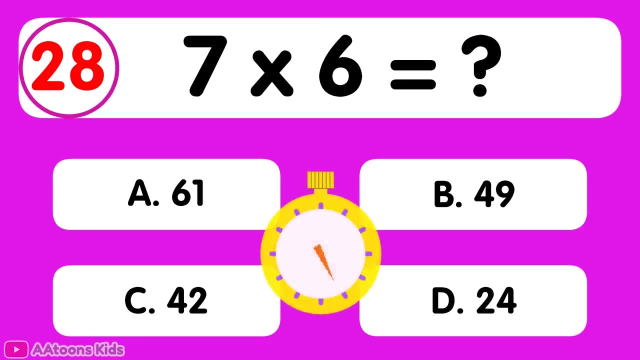 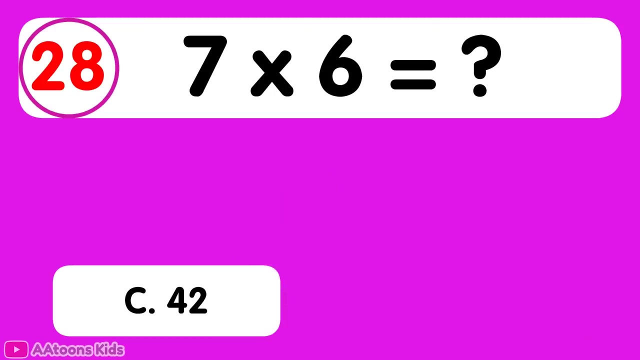 9. The answer was 1, 36. The answer was 2. 6 times 3 is equal to 36.. 7 times 6 is equal to 10 times 5 is equal to 6 times 6 is equal to. 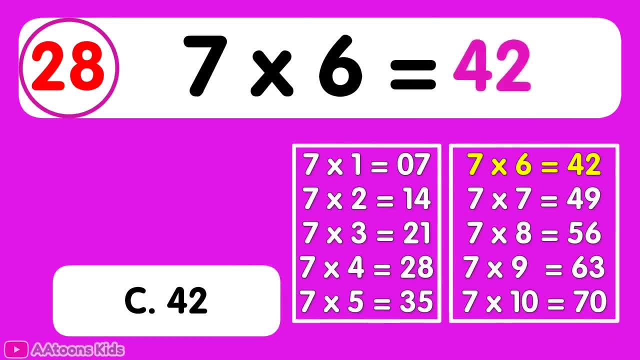 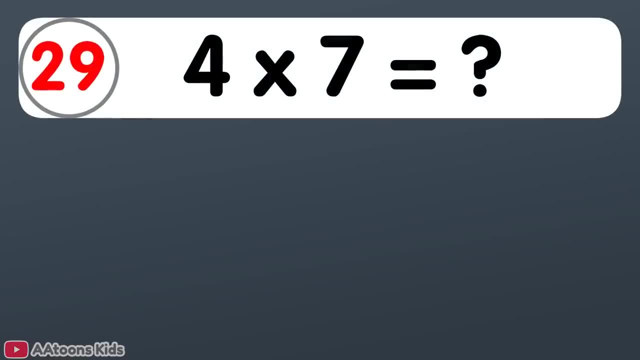 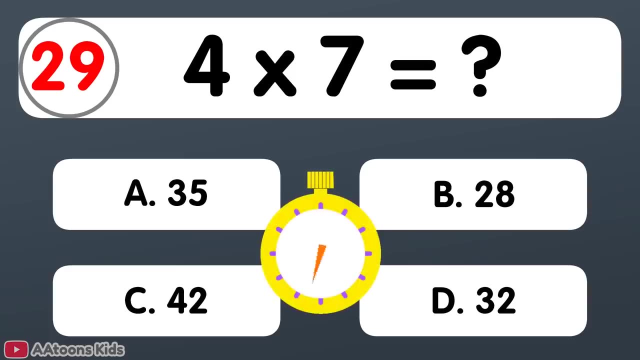 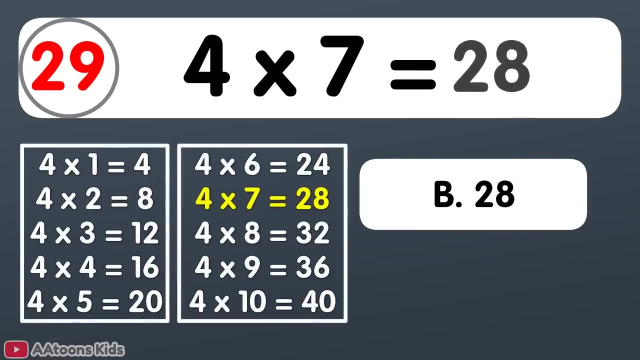 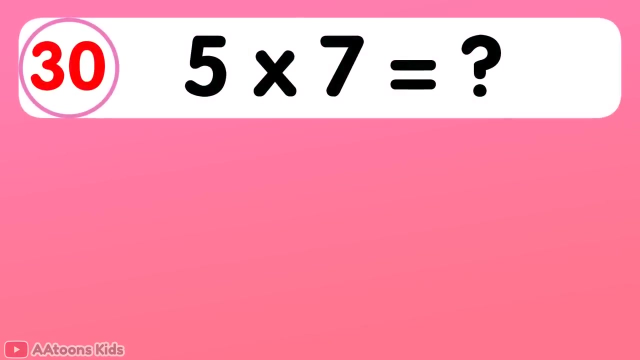 34.. 2 times 5 is equal to 47.. 6 times 6 is equal to 4. 6 times 5 is equal to times. 6 is 42. 4 times 7 is equal to 28. 4 times 7 is 28- 5. 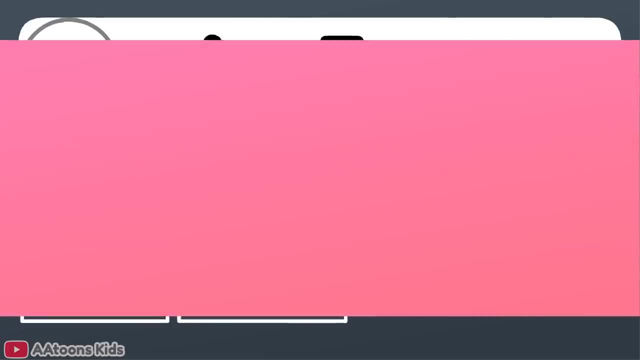 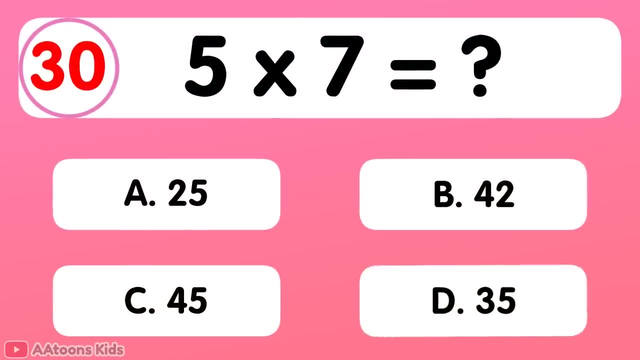 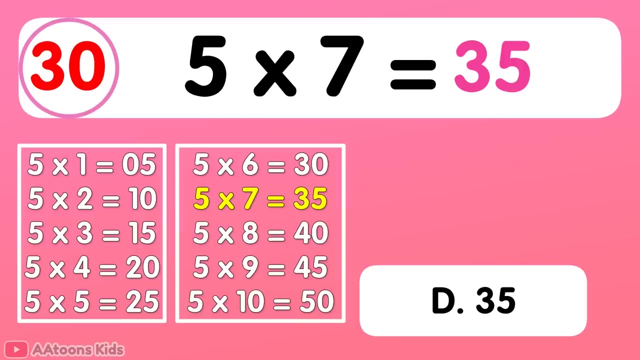 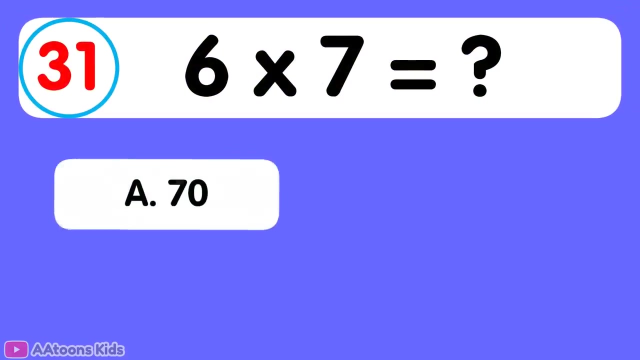 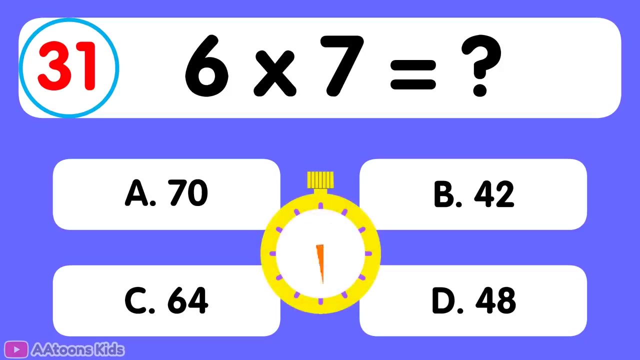 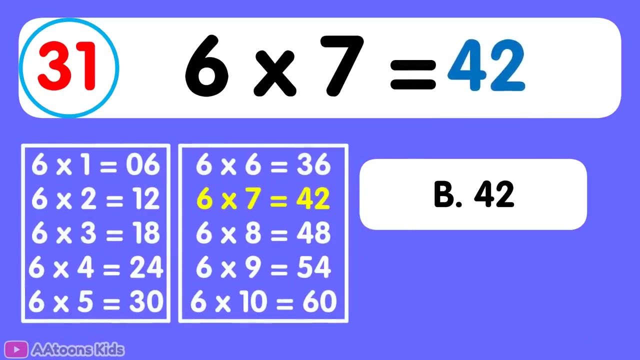 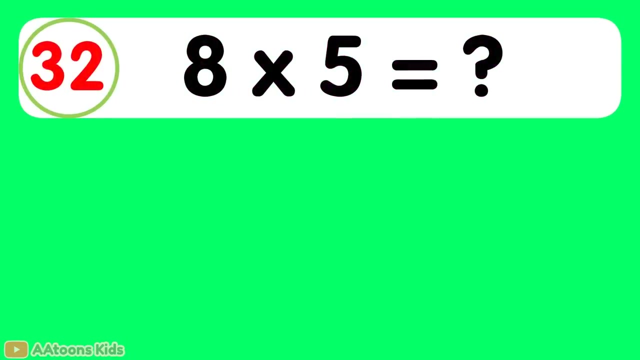 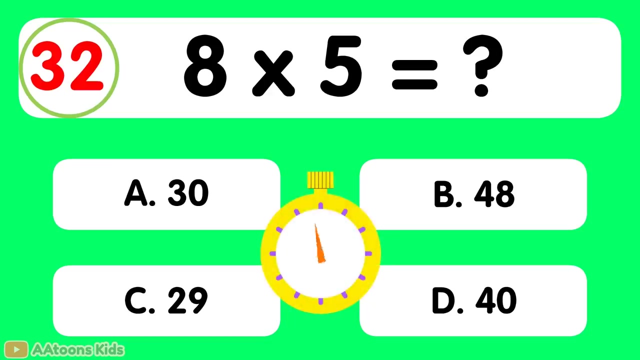 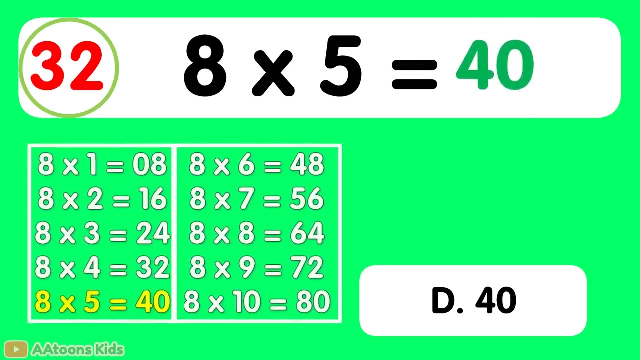 28.. 5 times 7 is equal to 3 times 7 is equal to 6 times 7 is equal to 23.. 35, 5 times 7 is 35. 6 times 7 is equal to 42,. 6 times 7 is equal to 42. 8 times 5 is equal to. 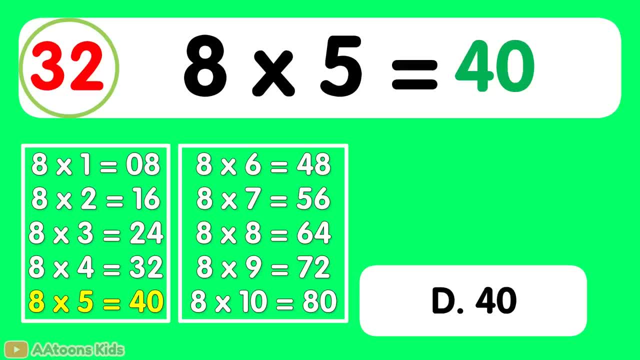 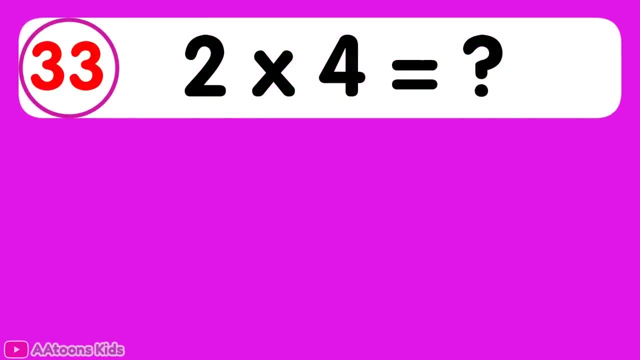 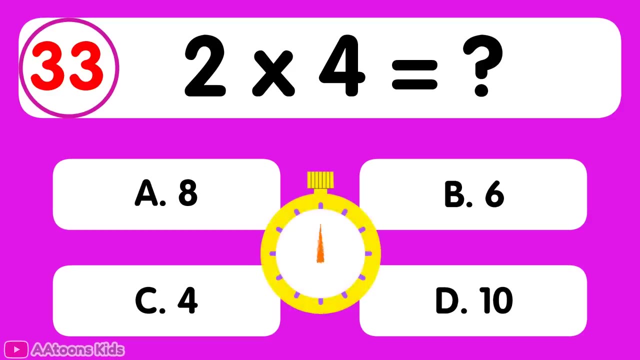 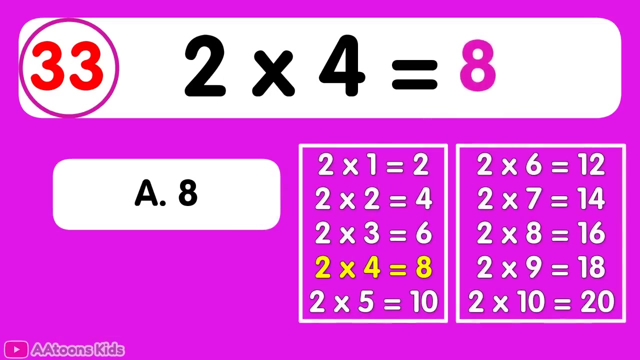 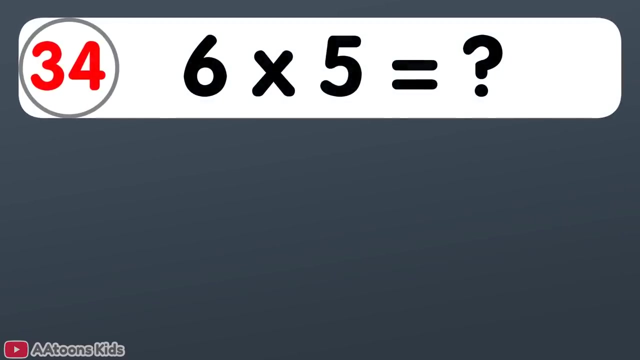 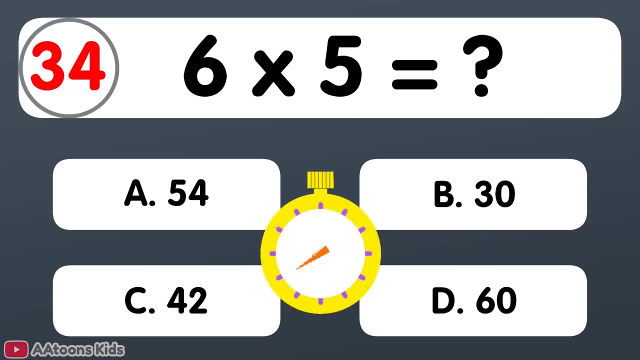 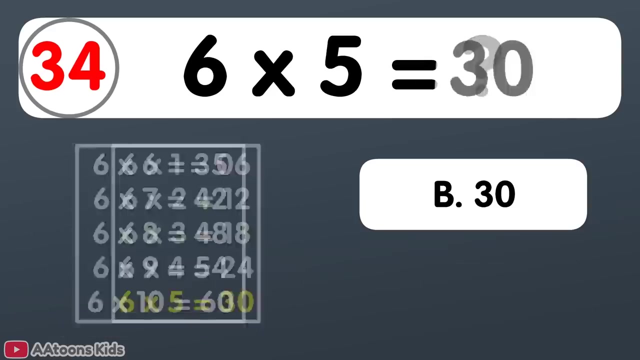 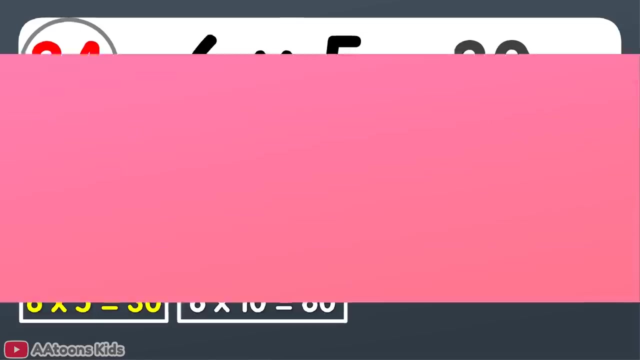 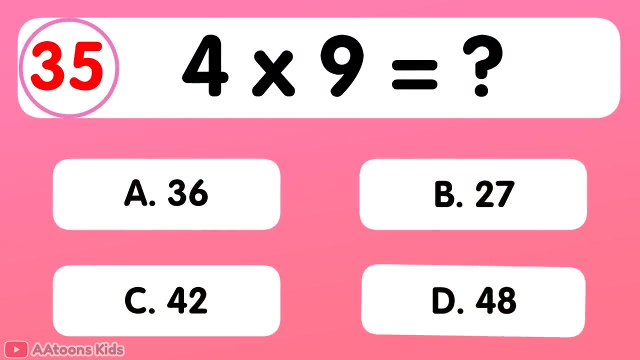 40. 8 times 5 is equal to 40. 2 times 4 is equal to 8,. 2 times 4 is 8. 6 times 5 is equal to 30. 6 times 5 is 30. 4 times 9 is equal to 36. 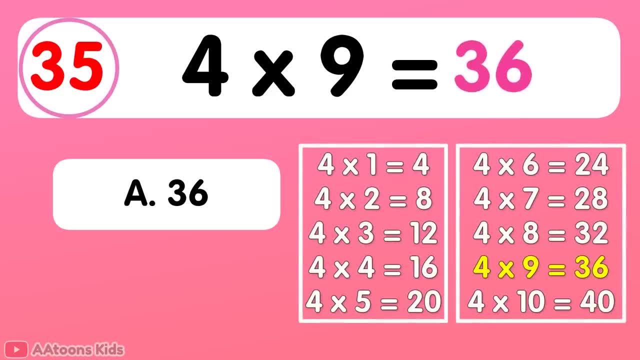 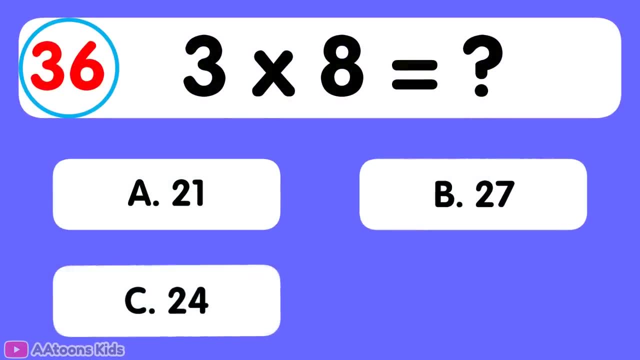 4 times 9 is 36. 3 times 8 is equal to 36. 4 times 9 is 36. 3 times 8 is equal to 36. 4 times 9 is equal to 36. 4 times 9 is equal to 36. 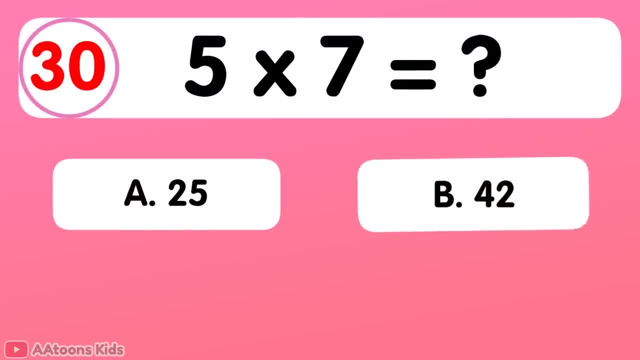 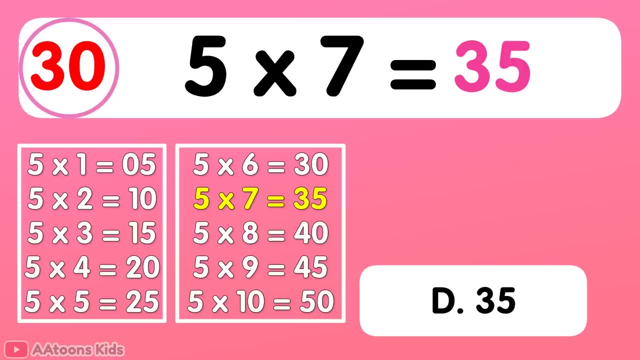 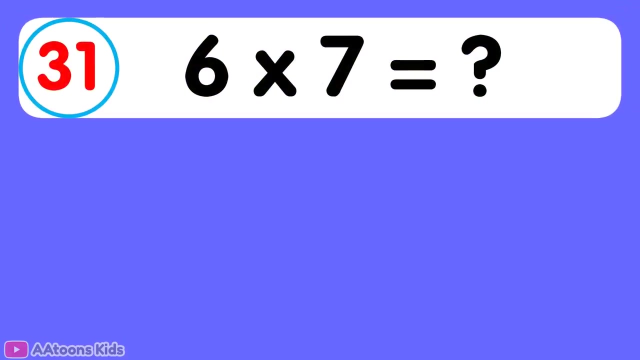 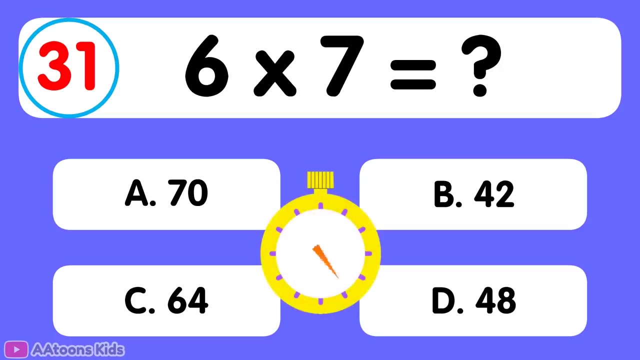 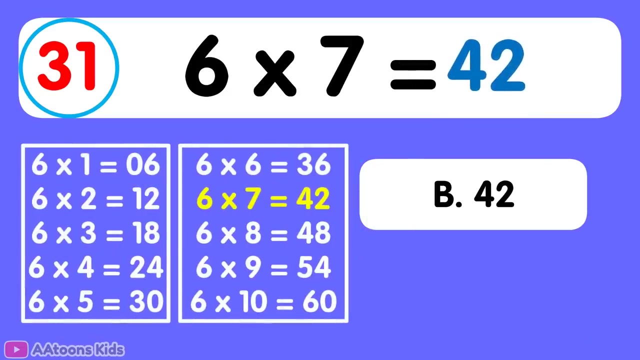 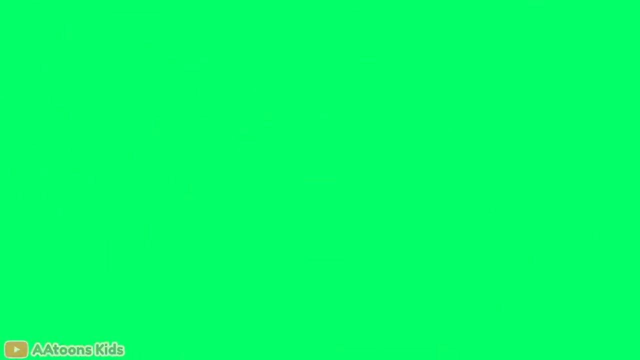 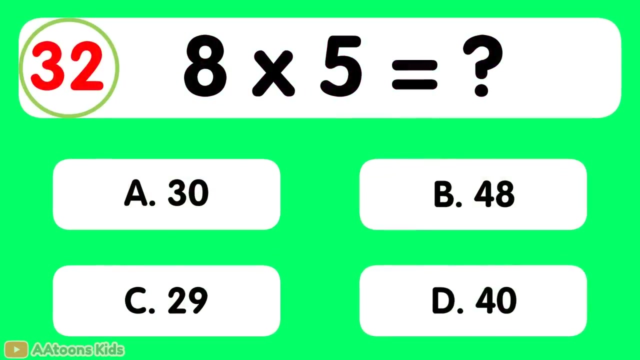 times 7 is equal to 35. 5 times 7 is 35. 6 times 7 is equal to 42. 6 times 7 is 42. 8 times 5 is equal to 8 times 5 is equal to 8 times 5 is equal to. 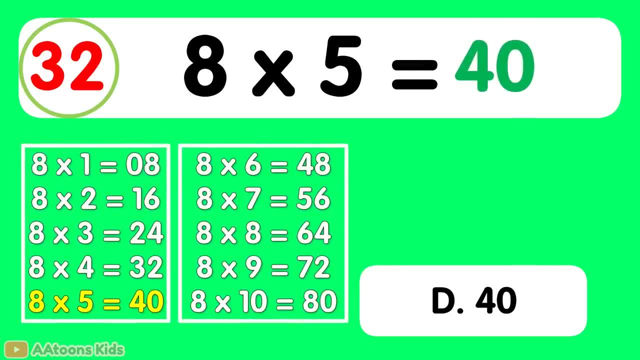 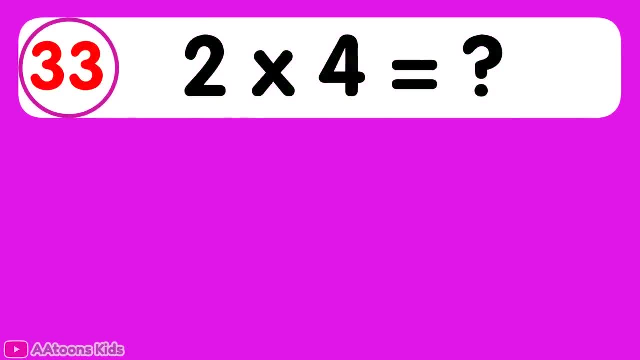 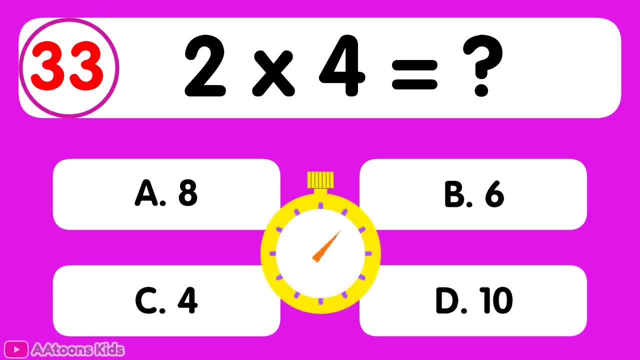 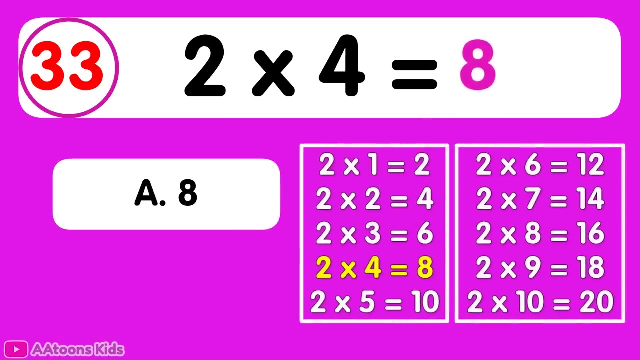 40. 8 times 5 is 40 2 times 4 is equal to 거죠. 8 2 times 4 is 8. 8 2 times 4 is 8. 8 2 times 4 is 8. 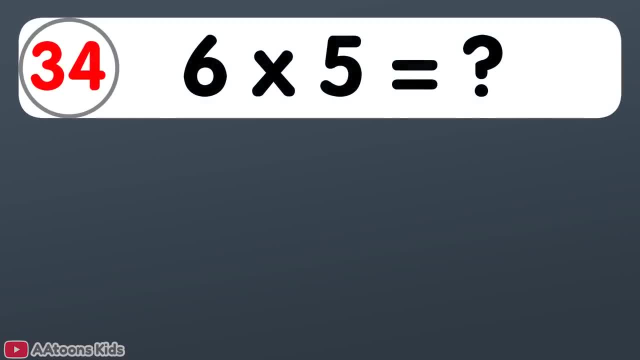 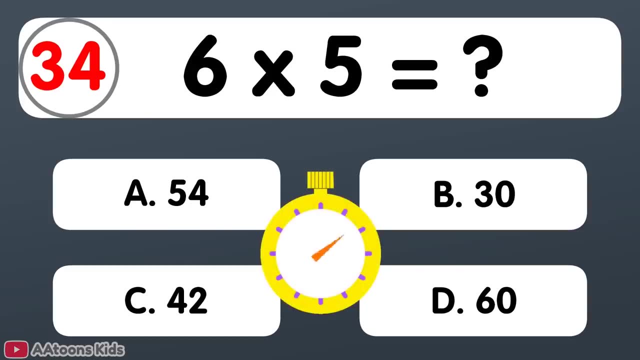 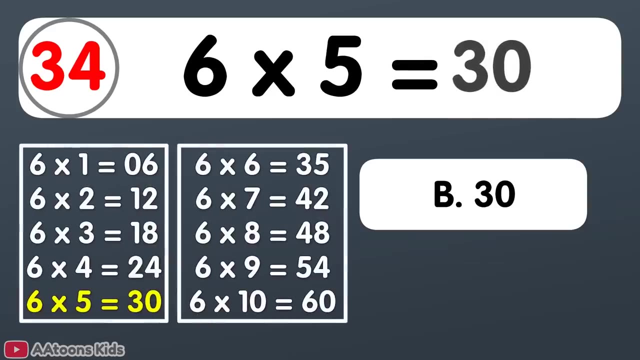 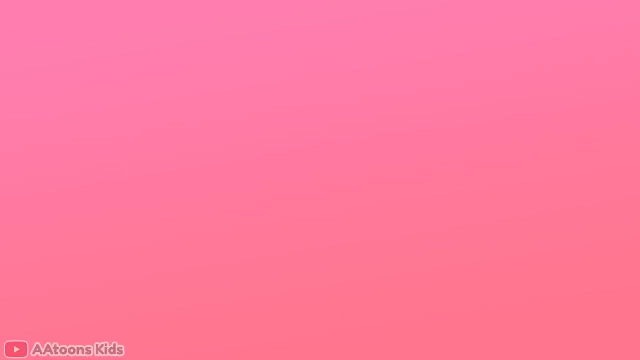 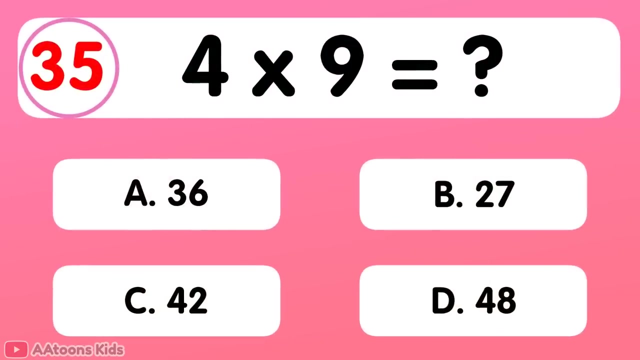 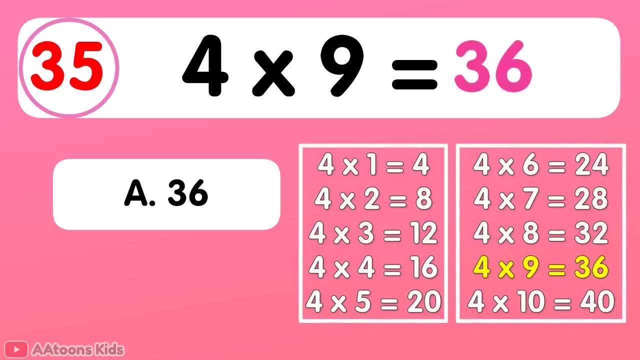 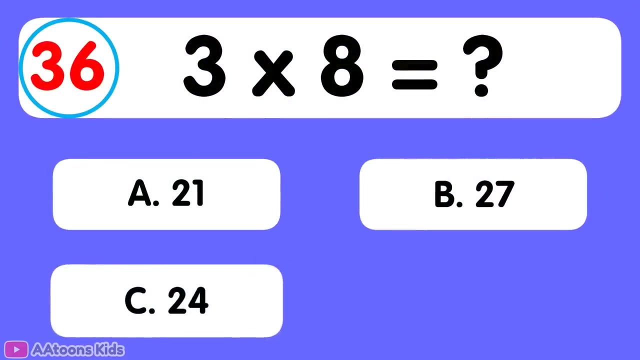 6 times 5 is equal to 30. 6 times 5 is equal to 30. 4 times 9 is equal to 36. 4 times 9 is equal to 36. 3 times 8 is equal to 3 times 8 is equal to.